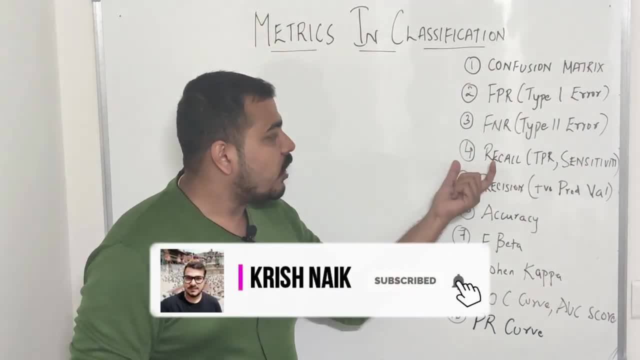 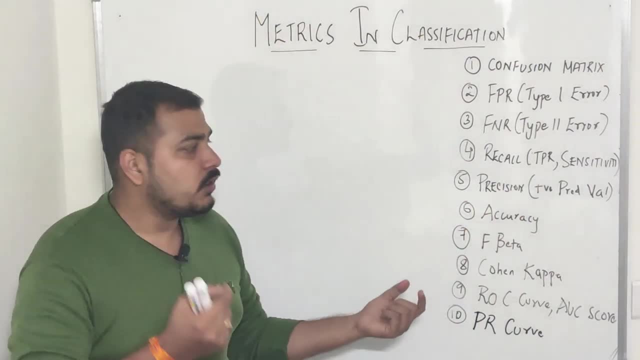 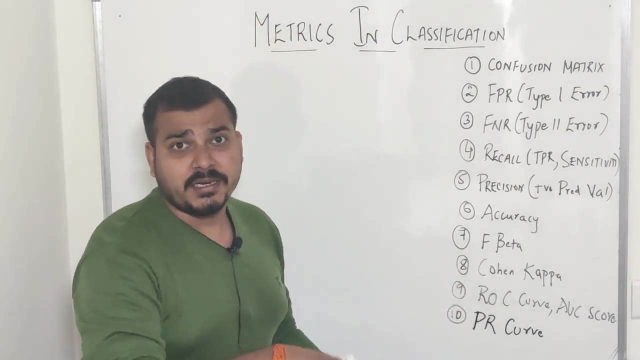 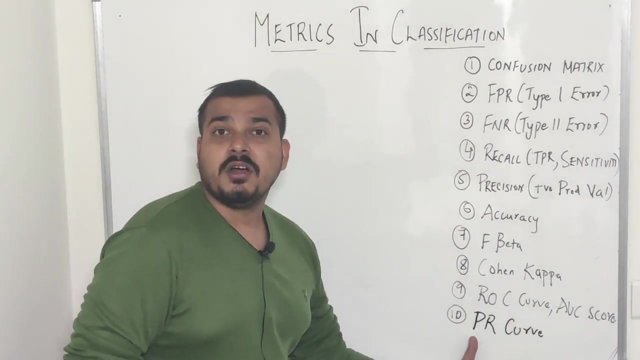 Then we'll understand about type one error, type two error. Then we have concepts like recall, which is also called as true positive read. Then we'll discuss about precision, which is also called as positive prediction value. Okay, then we'll understand about F, beta. And in the next part, in the next video, we'll basically be understanding about Cohen, kappa, ROC curve, AUC score and something called as PR curve. There are two more metrics again which I'll discuss in the part two, because I do not have 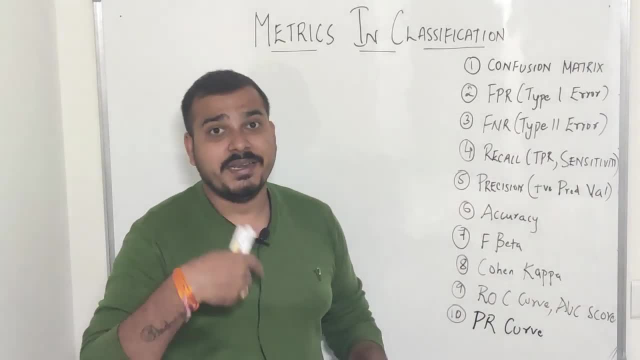 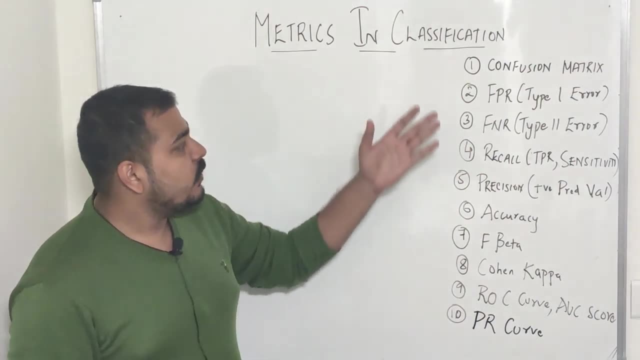 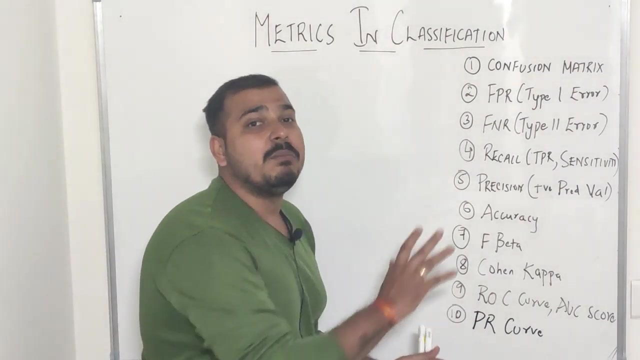 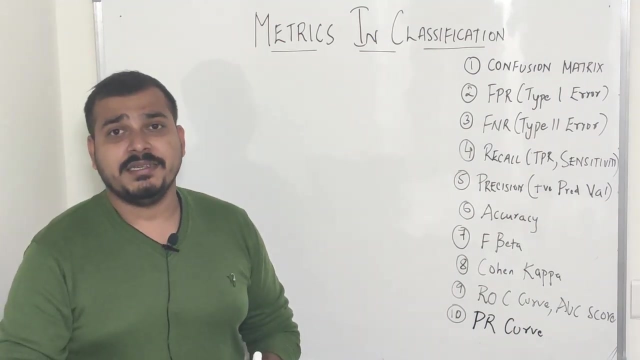 had space to write it down, So we'll just be discussing about that in our next part two. In the part three, I'll try to implement a problem statement, considering an imbalanced data set, and I'll try to apply all this particular metrics and I'll show you that how the accuracy will look like. So make sure, guys, you watch this particular video completely and make sure that you understand things. Okay, the reason why I'm saying, even though you are a very, very good data scientist and you know how to actually use a machine learning algorithm with respect to your data, but if you're not, 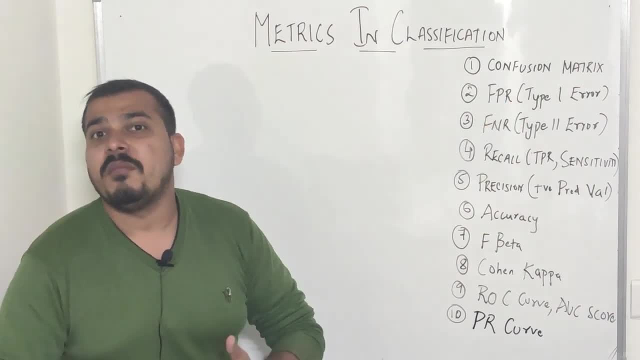 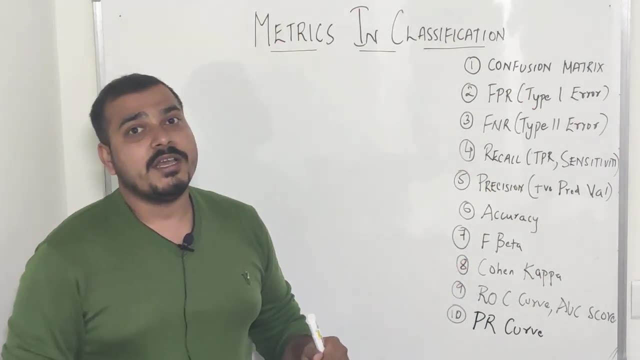 using the correct kind of metrics to find out how good your model is, then it is completely a waste of time, You know, because if you have not selected the right metrics and then you have deployed your model to the production right, you'll be able to see that because of the metrics, because of the wrong metrics that you have chosen, you have chosen that will actually give you a very, very bad accuracy again when the model is actually deployed in the production. So let us go ahead and try to understand the metrics And in this particular video I'll be making like a story. 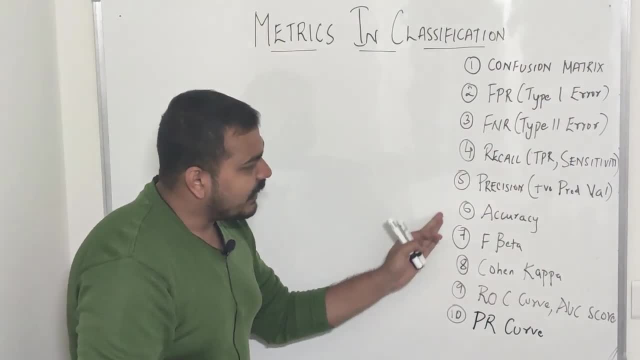 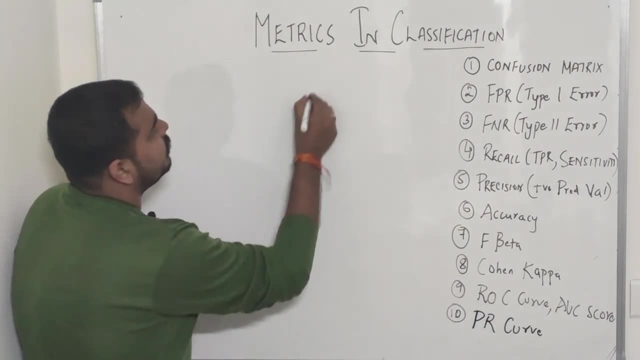 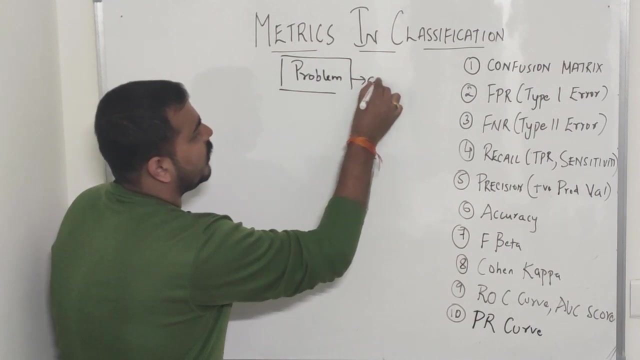 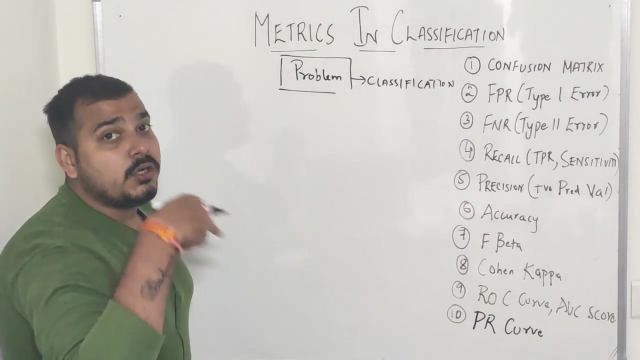 Okay, so part one will just be like a story And then I'll continue and I'll explain you each and every metrics over here. Now understand one thing: that suppose we have a problem statement, So this is a problem statement, specifically a classification problem statement. Okay, classification problem statement. Now, in classification problem statement, right, there are two ways how you can solve the classification problem. One way is basically through: 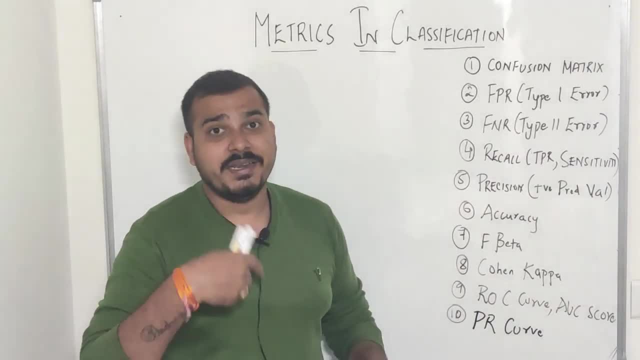 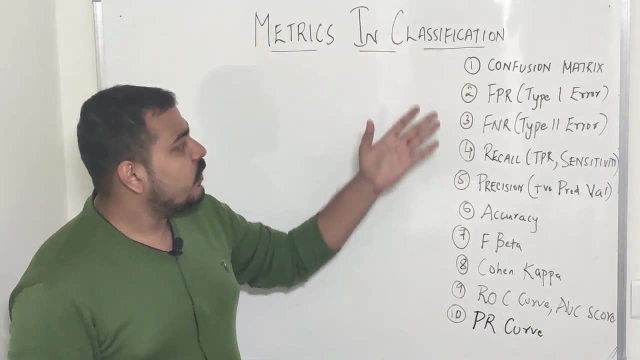 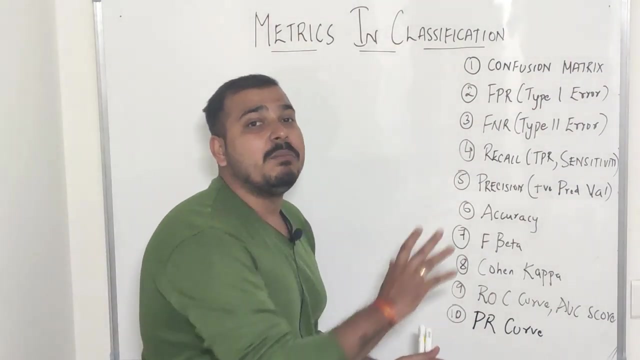 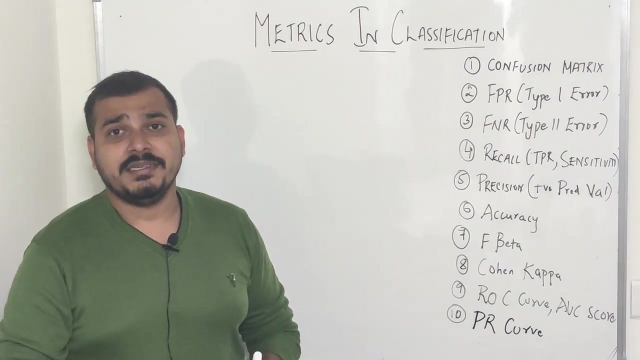 had space to write it down, So we'll just be discussing about that in our next part two. In the part three, I'll try to implement a problem statement, considering an imbalanced data set, and I'll try to apply all this particular metrics and I'll show you that how the accuracy will look like. So make sure, guys, you watch this particular video completely and make sure that you understand things. Okay, The reason why I'm saying, even though you are a very, very good data scientist and you know how to actually use a machine learning algorithm with respect to your data, But if you're 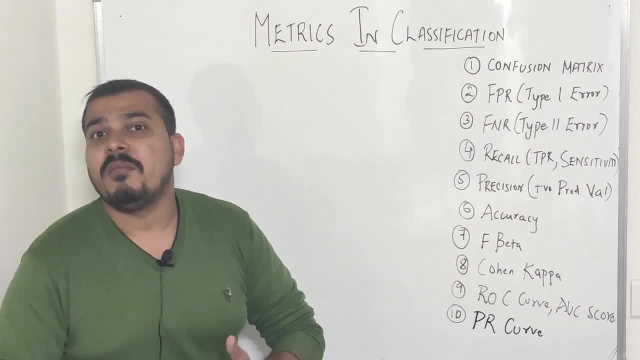 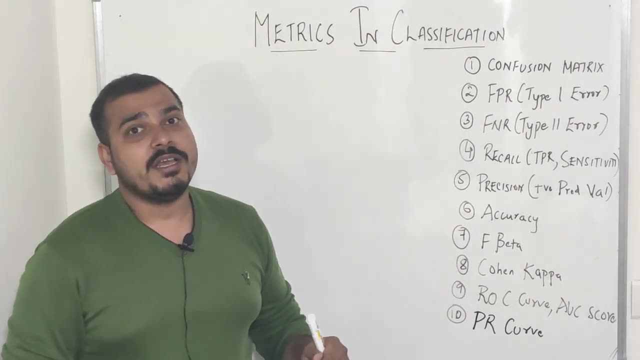 not not using the correct kind of metrics to find out how good your model is, then it is completely a waste of time, you know, because if you have not selected the right metrics and then you have deployed your model to the production right, you'll be able to see that because of the metrics, because 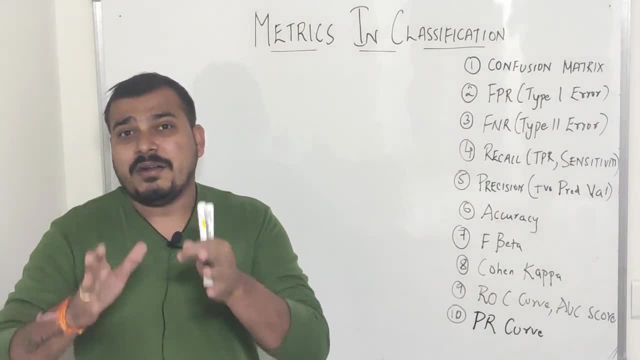 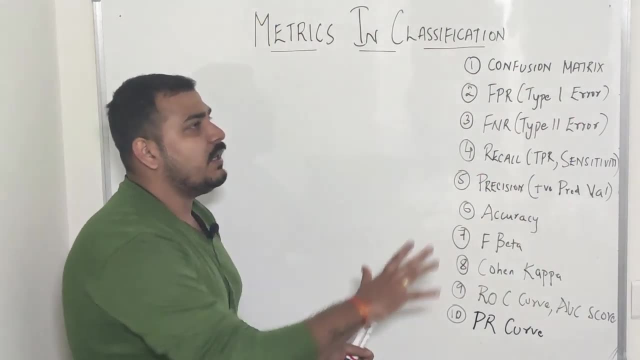 of the wrong metrics that you have chosen. you have chosen that will actually give you a very, very bad accuracy again when the model is actually deployed in the production. so let us go ahead and try to understand the metrics, and in this particular video i'll be making like a story. 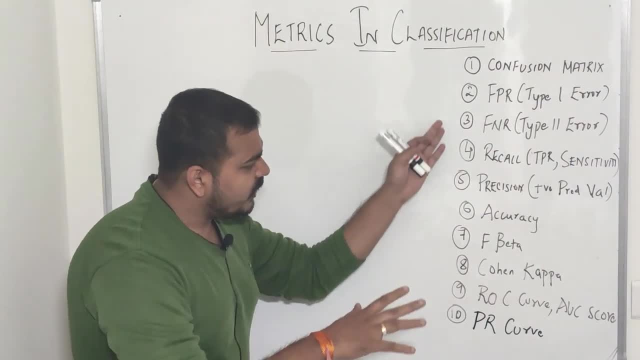 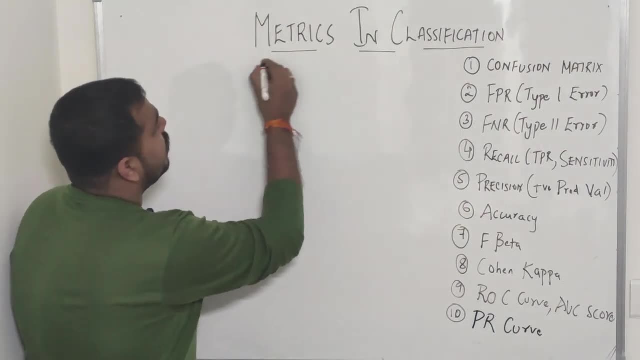 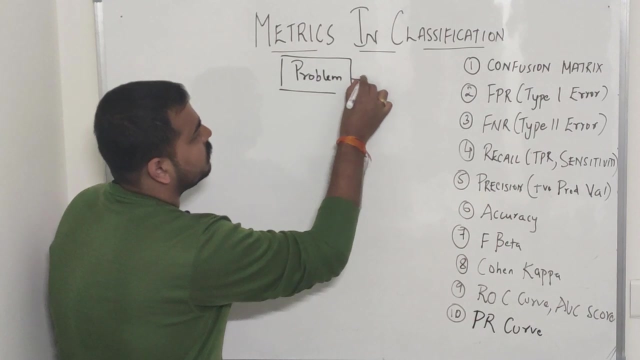 okay, so part one will just be like a story and then i'll continue and i'll explain you each and every metrics over here. now understand one thing, guys: suppose we have a problem statement. so this is a problem statement, specifically a classification problem statement. okay, classification problem. 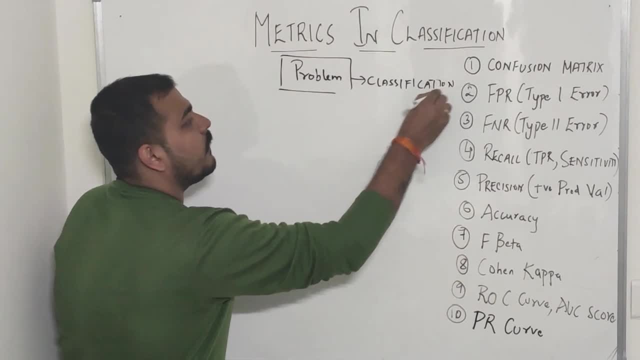 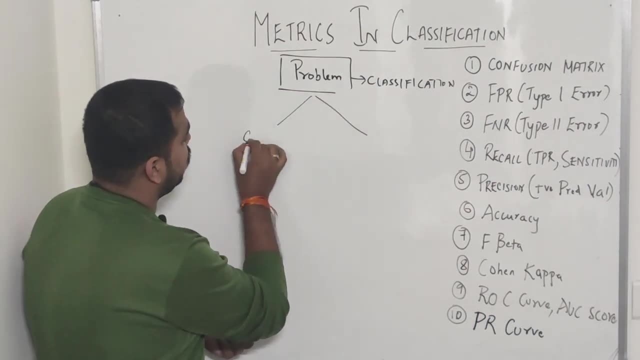 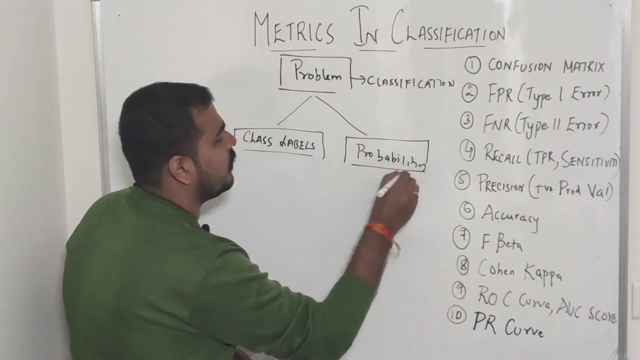 statement now in classification problem statement. right, there are two ways how you can solve the classification problem. one way is basically through class labels. suppose you want to predict class labels, okay. the next way is through probabilities. probabilities now, suppose if let me just consider a binary classification, in a binary classification, i know there will be. 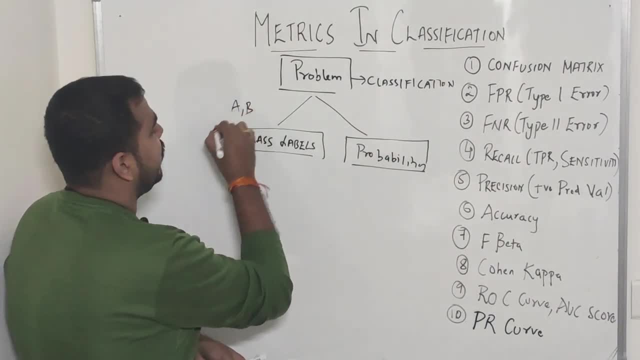 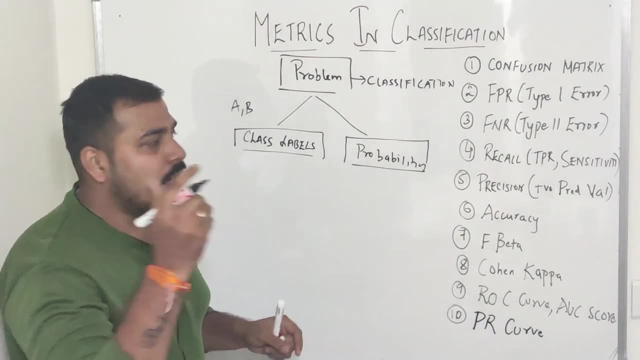 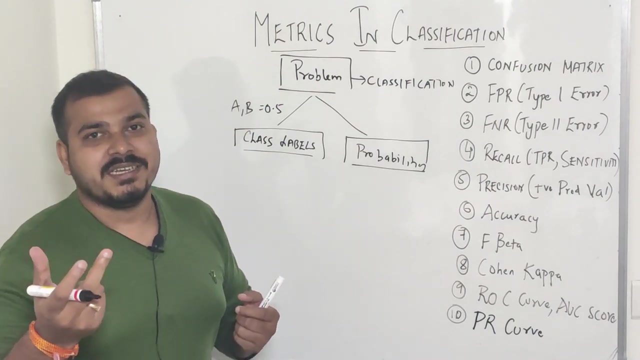 two different classes, a or b. suppose this is my a or b, so my output will either be a or b. okay, by default the threshold value will be taken as 0.5. what does this basically mean? suppose i am predicting with some of my machine learning model, like logistic regression by default, if i predict if it is greater than 0.5. 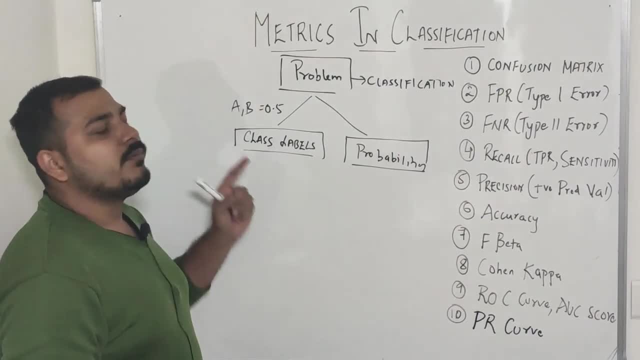 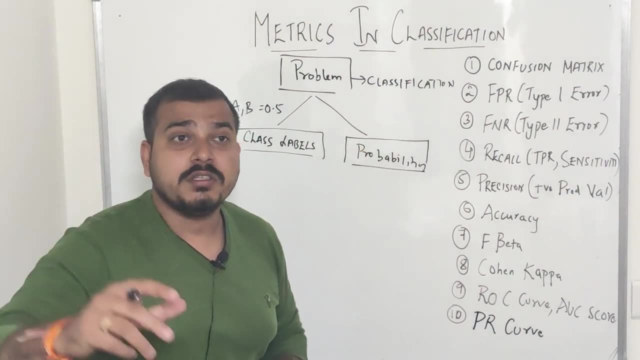 then it will become a b class. if it is less than 0.5, then it becomes a a class. i mean less than or equal to 0.5, then it will become a a class. but in case of probabilities here we have to also find: 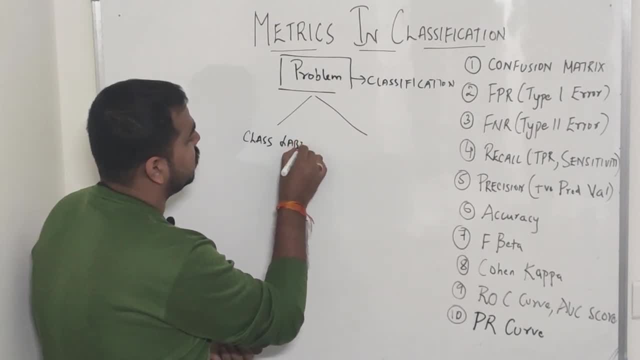 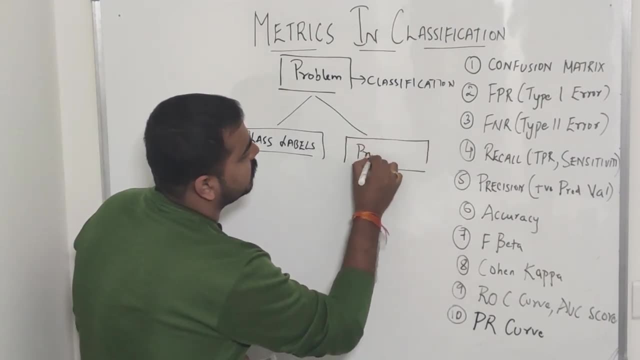 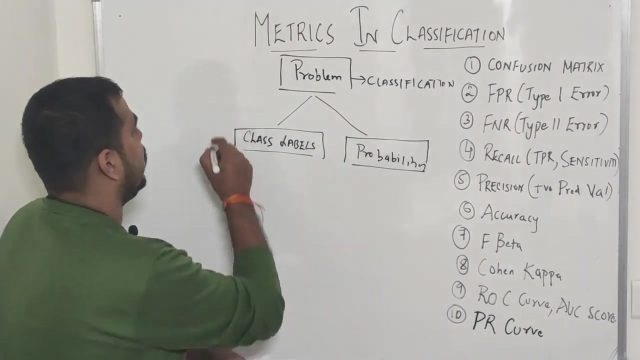 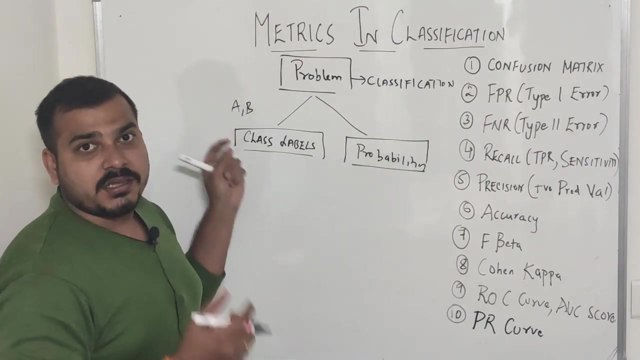 class labels. Suppose you want to predict class labels. Okay, the next way is through probabilities. Probabilities Now, suppose I. if let me just consider a binary classification. In a binary classification, I know there will be two different classes, A or B. Suppose this is my A or B, So my output will either be A or B. Okay, by default, the threshold value will be taken as 0.5.. What does this basically mean? 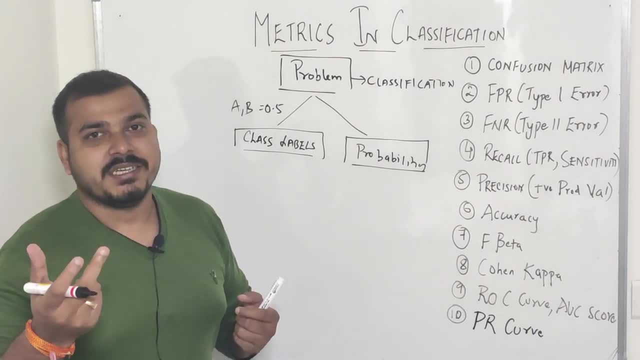 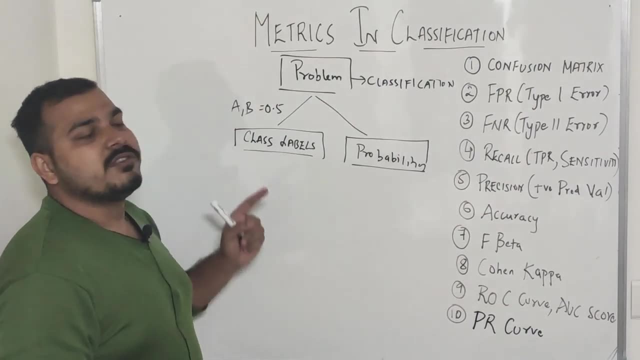 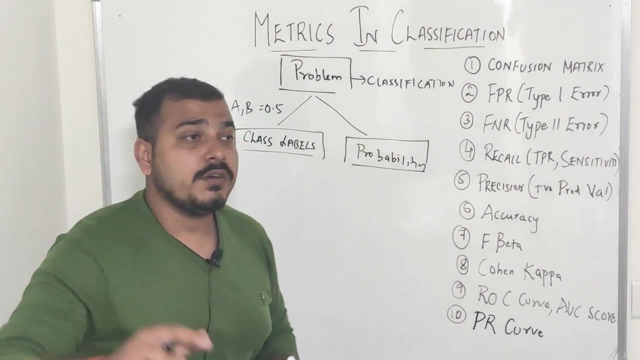 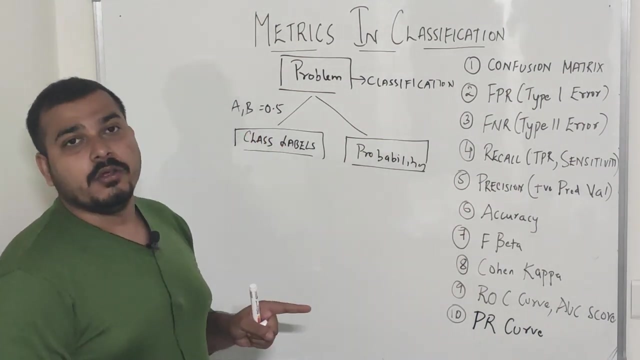 I am predicting with some of my machine learning model, like logistic regression, By default. if I predict, if it is greater than 0.5, then it will become a B class. If it is less than 0.5, then it becomes a A class. I mean less than or equal to 0.5, then it will become a A class. But in case of probabilities, here we have to also find out the class labels, how we have to basically select the right threshold value, which is this P value? Okay, I'll not say P value, but I'll instead say some threshold value in some of the healthcare sectors. 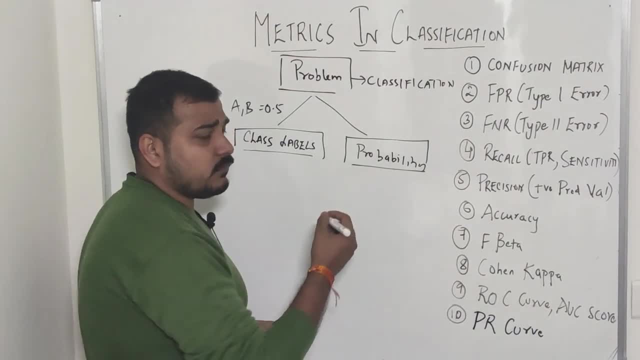 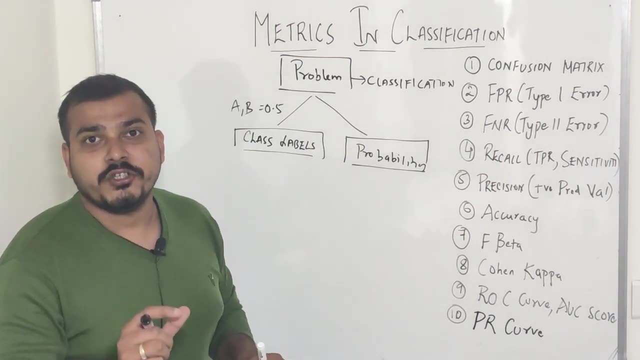 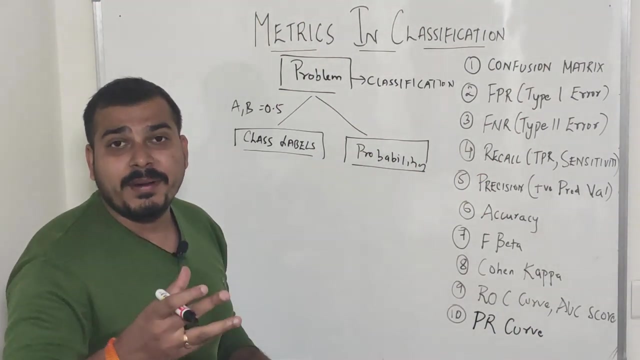 This threshold value may decrease. You will be saying that suppose if a person is having cancer or not. at that time, this threshold value should be chosen in a proper way. If it is not chosen in a proper way, the person who is having cancer will be missed out, Right? So in probabilities, we will be discussing, and in probabilities, what all we have. we have basically ROC curve, AUC curve, AUC score and PR curve, which we'll be discussing in the part two. In the part one, we'll be focusing more on this class labels. 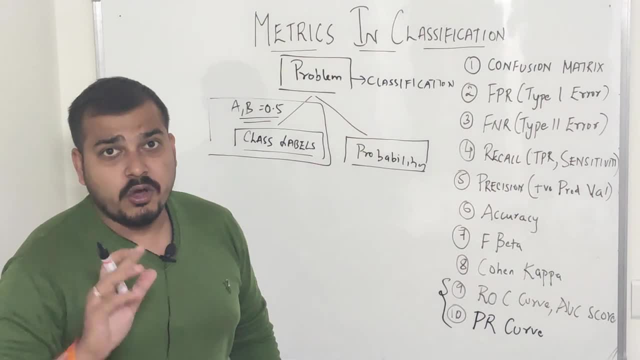 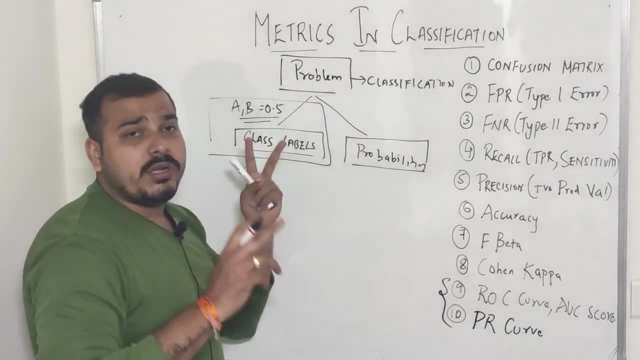 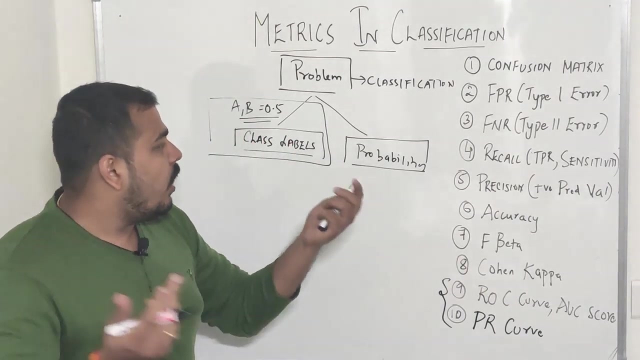 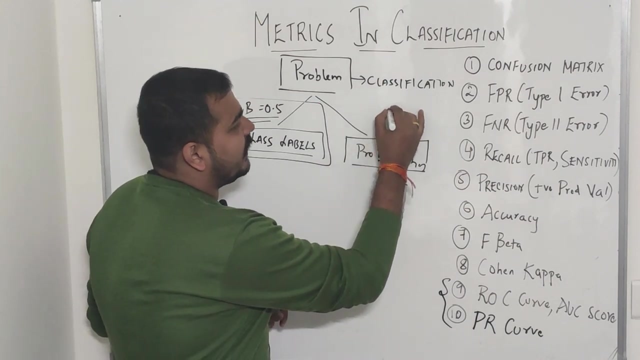 Where our default probability is 0.5.. Okay, so I hope you are getting it right. So understand that thing. if we have a classification problem, usually what we do is that they have two types of problem statements over here. with respect to the class labels, we need to find out what. what is the output of that particular record? or based on probabilities, where we have to first of all find out a threshold value. Okay, in logistic regulation, I may find out that the threshold value may be 0.3, maybe 0.4. That basically means that if my output is less than or equal to 0, I will get 0.5. 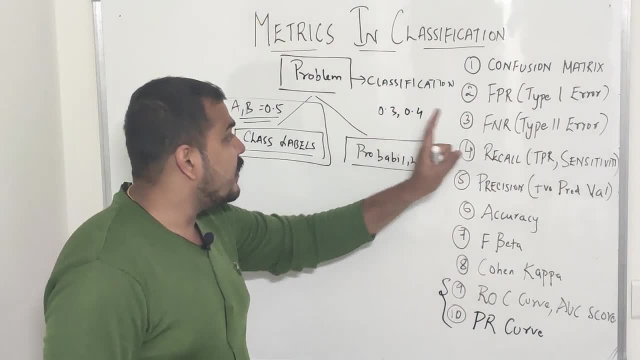 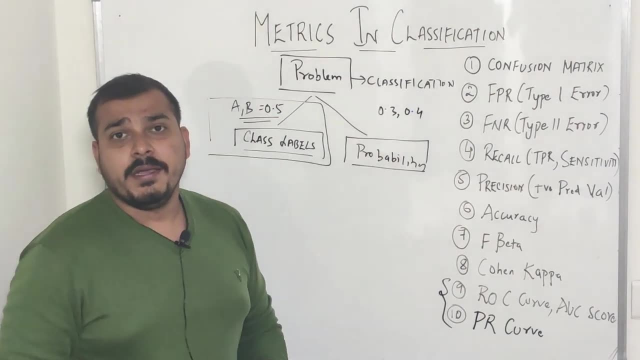 or equal to 0.4, it becomes class a. if my output is greater than 0.4, then it becomes class b. right, and this i'll be showing you how you can actually find out with the help of roc curve and pr curve. okay, so that will come in the part two. now let us go ahead. one more thing now over. 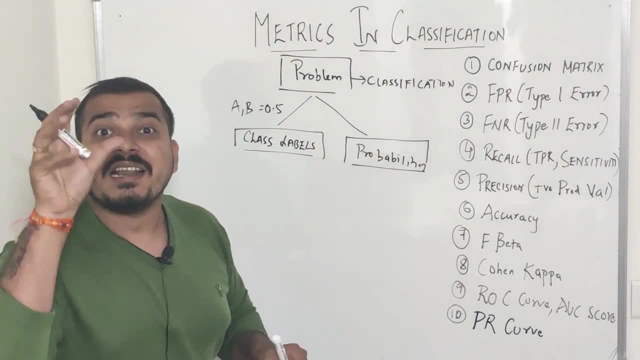 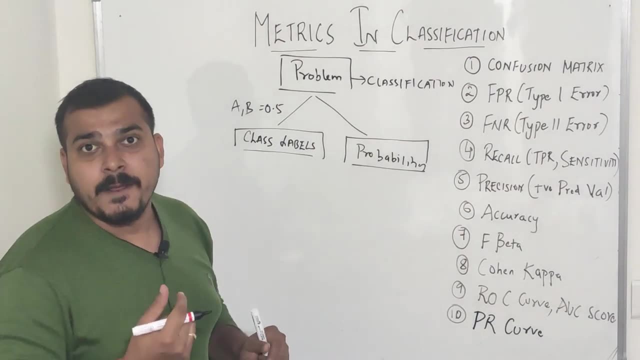 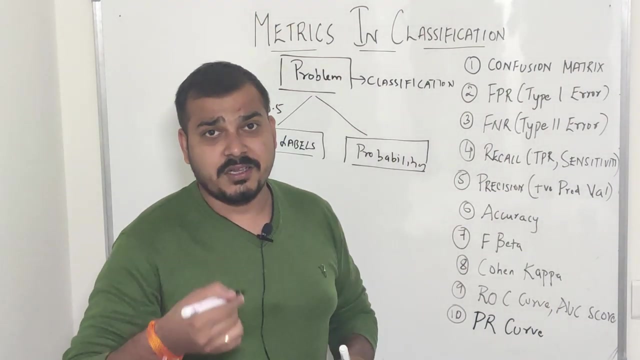 out the class labels, how we have to basically select the right threshold value, which is this, a p value, but i'll instead say some threshold value. in some of the health care sector, this threshold value may decrease. you will be saying that suppose, if a person is having cancer or not. 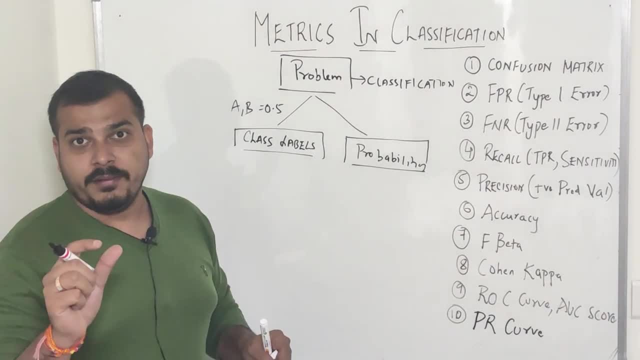 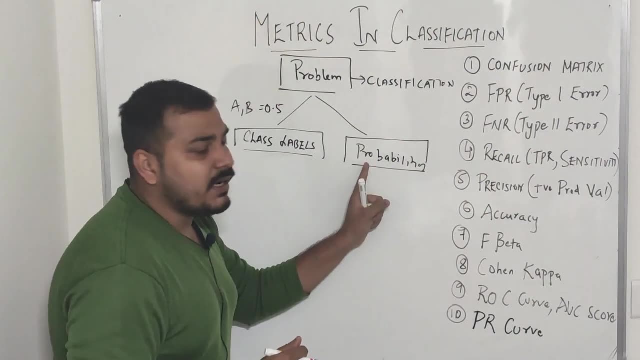 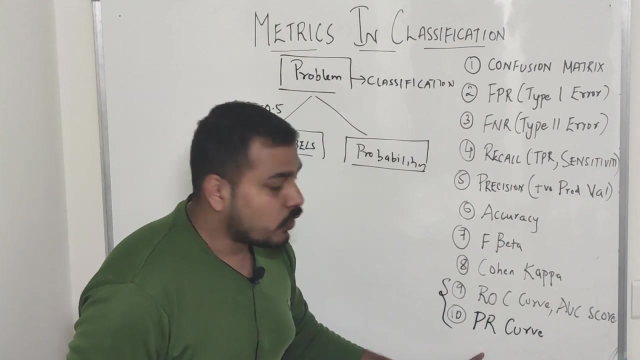 at that time, this threshold value should be chosen in a proper way. if it is not chosen in a proper way, the person who is having cancer will be missed out right. so in probabilities, we will be discussing, and in probabilities, what all we have? we have basically roc, curve, auc, curve, auc, score and pr. 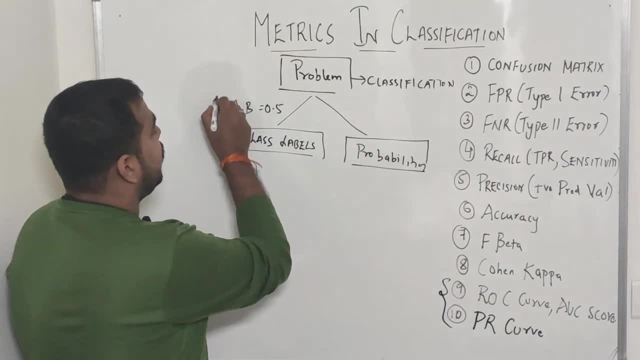 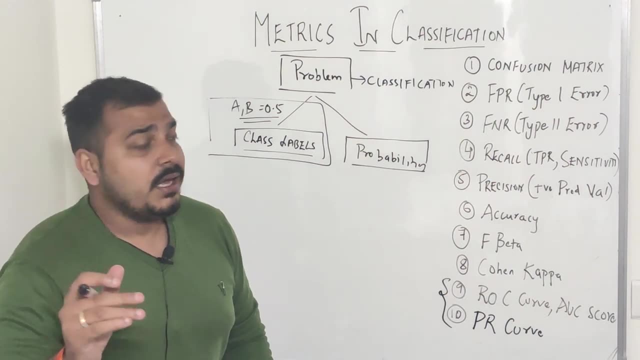 curve, which we will be discussing in the next video. so thank you for watching and i will see you in the next video in the part two. in the part one, we'll be focusing more on this class labels, where our default probability is 0.5. okay, so i hope you are getting it right. so understand that thing. if we have a 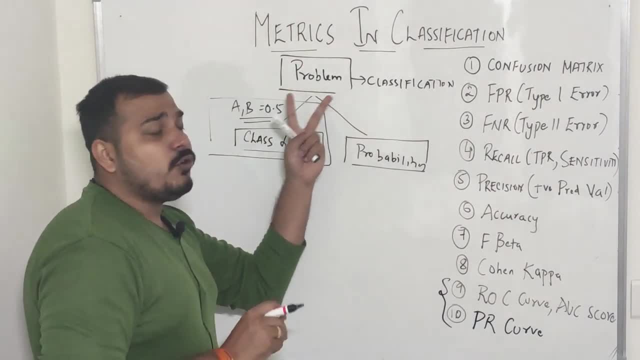 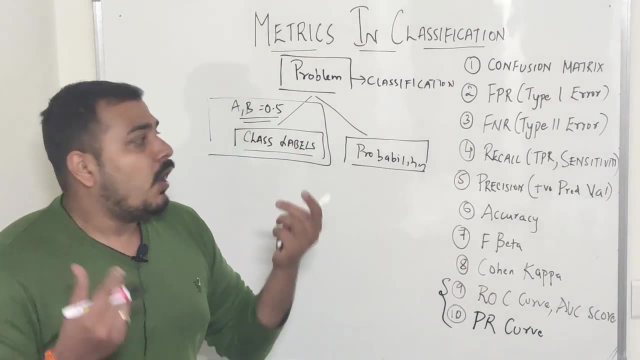 classification problem. usually what we do is that they have two types of problem statements over here. with respect to the class labels, we need to find out what. what is the output of that particular record? or based on probabilities, where we have to first of all find out a threshold value. okay, in. 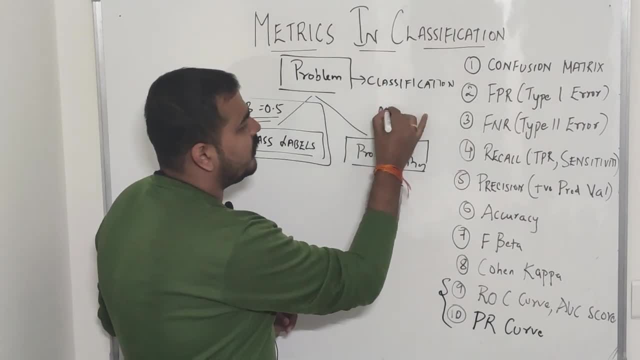 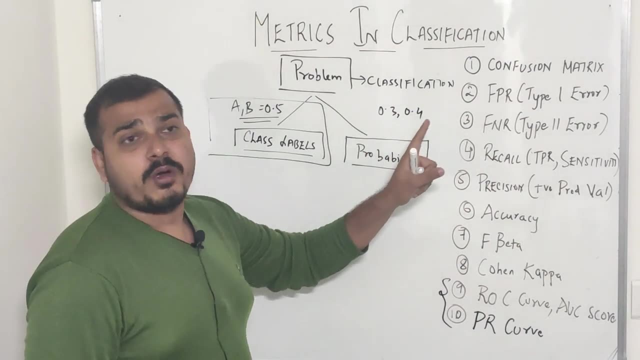 logistic regression, i may find out that the threshold value may be higher than or equal to 0.5. may be point three. may be point four. that basically means that if my output is less than or equal to 0.4, it becomes class a. if my output is greater than 0.4, then it becomes class b. right, and this. 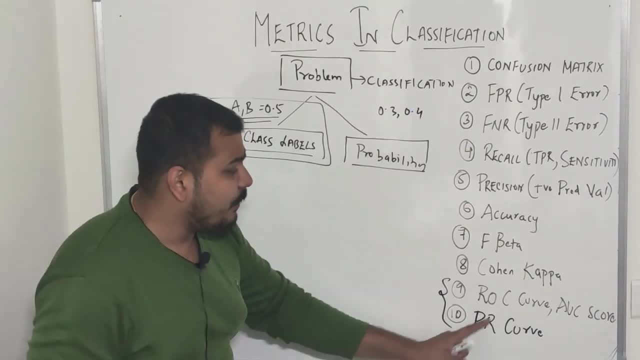 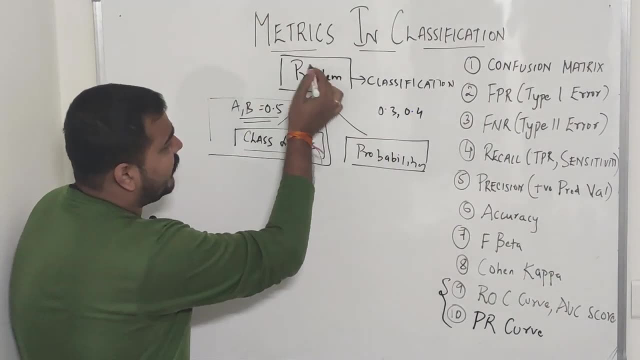 i will be showing you how you can actually find out with the help of roc curve and pr curve. okay, so that will come in the part two. now let us go ahead. one more thing now, over here. now, with respect to this problem statement, we have two problem statement: based on the output, okay. based on the. 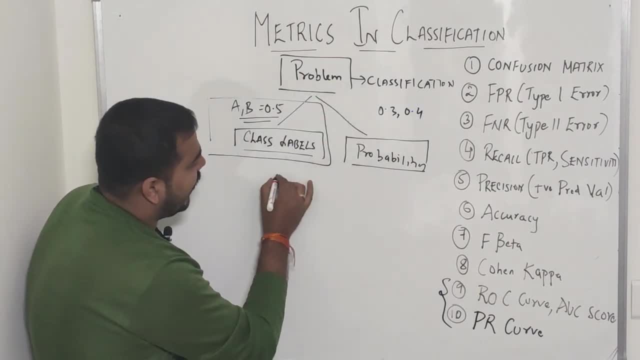 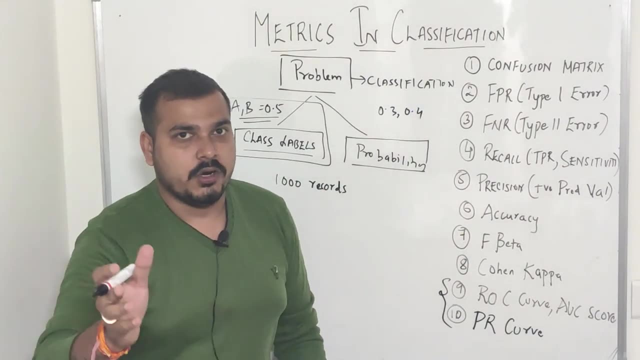 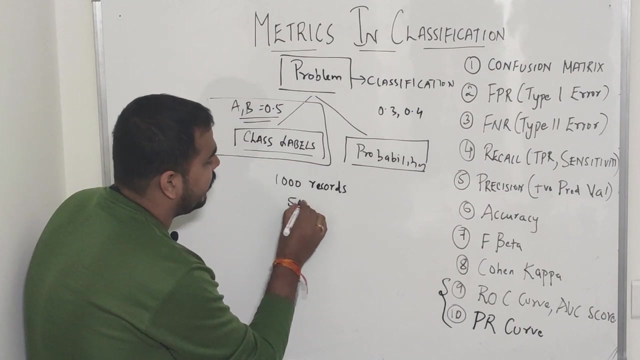 output. suppose in in this particular problem, statement f is the same value as the output of have thousand records. okay, I have thousand records. okay. now, with respect to thousand records, suppose this is a binary classification problem. that basically means: suppose I have 500- yes, that basically 500 records, which has yes as an output, and I have 500 no as my other output, or I? 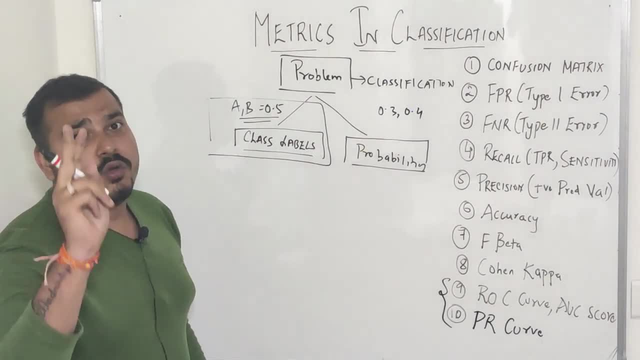 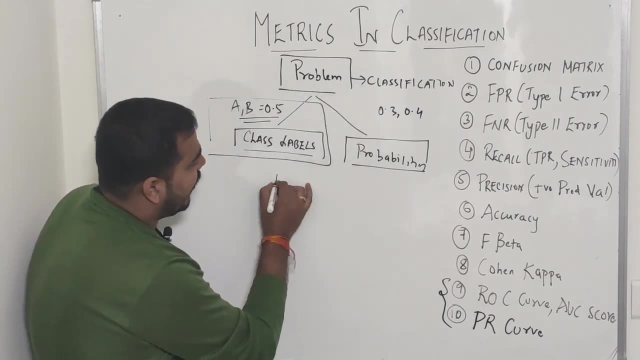 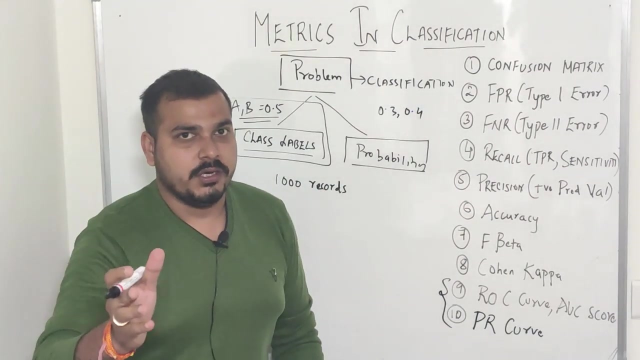 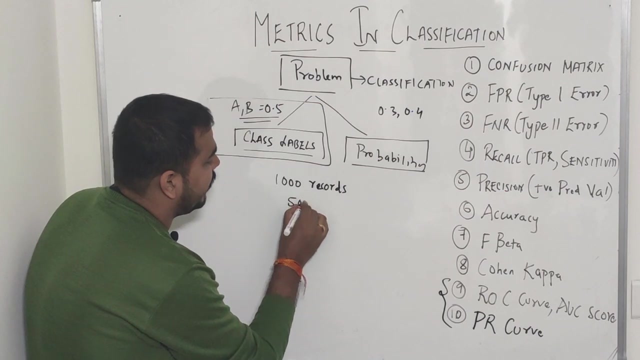 here. now, with respect to this problem statement, we have two problem statement: based on the output: okay, based on the output. suppose, in in this particular problem statement, i have thousand records. okay, i have thousand records. okay. now, with respect to thousand records, suppose this is a binary classification problem. that basically means: suppose i have 500. yes, that basically 500. 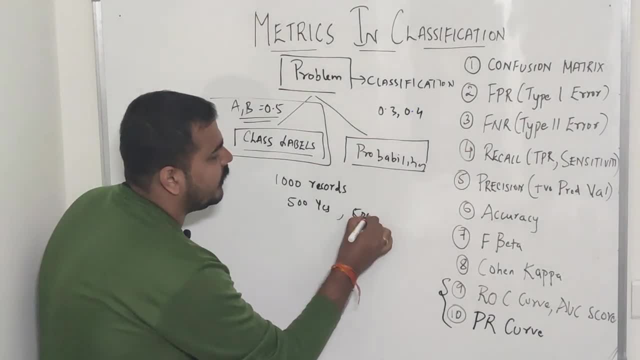 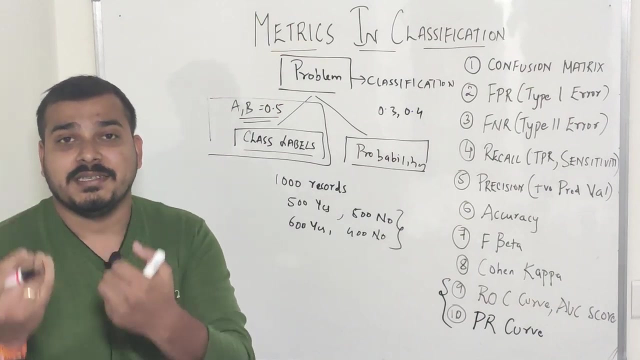 records which has yes as an output and i have 500 no as my other output, or i may have 600 yes or 400 no right now. in this case, what i can suggest is that this looks like an. this looks like a balanced data set. okay. balanced data set basically means: 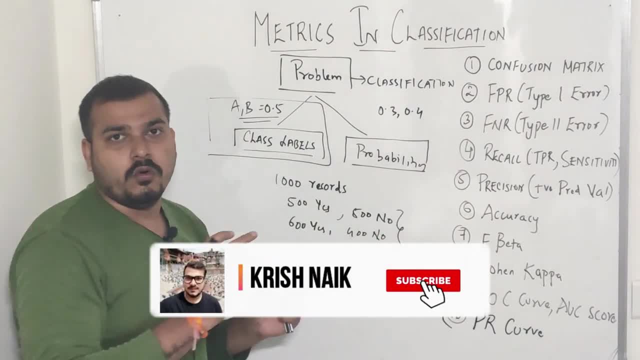 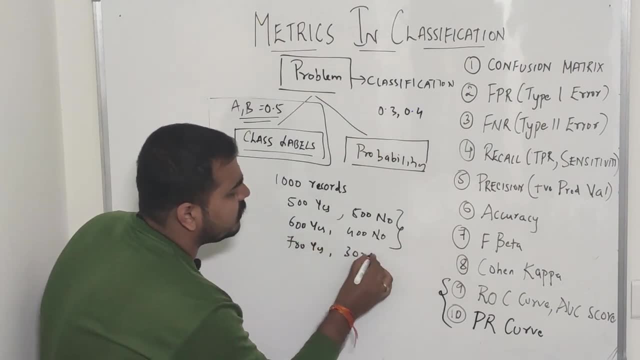 that, yes, you have almost same number of yes and same number of no, so both the output labels are almost same. similarly, if you could take 700 yes and 300 no, this is also fine. this looks like a balanced data set. okay, now understand one thing, guys, why, why i'm saying balanced data set over. 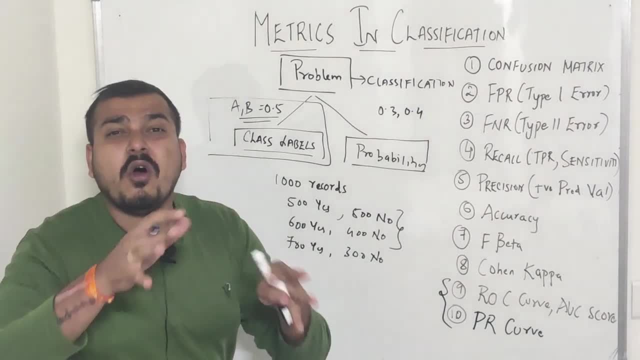 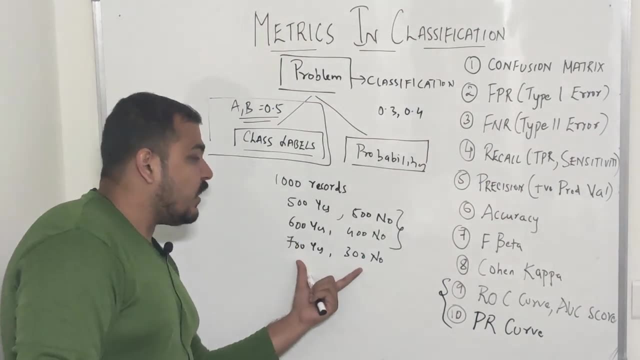 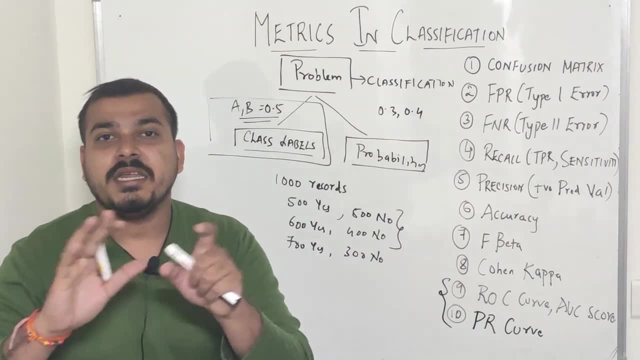 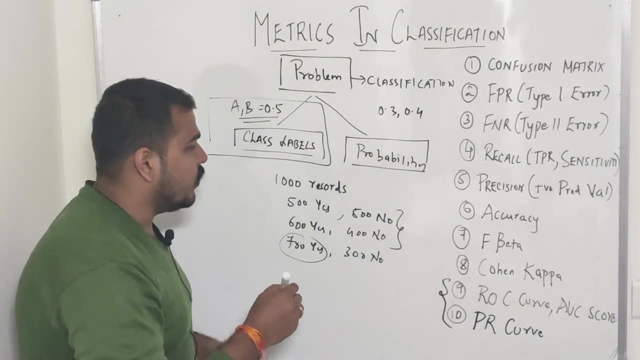 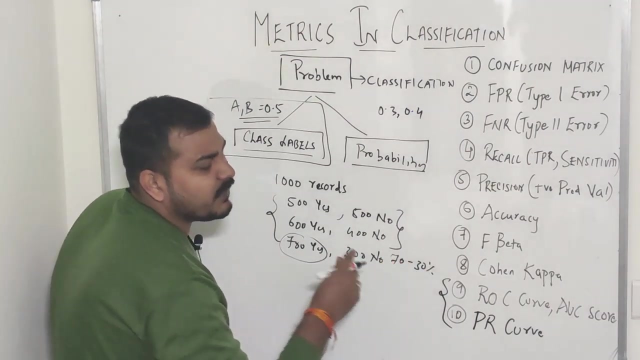 provide this kind of data points to our machine learning algorithm. my machine learning algorithm will not get biased based on the maximum number of output, okay. but if we have scenarios where in our data set ranges- and this is basically 70 to 30, right, 70 to 30, basically 70 to 30 ratio. 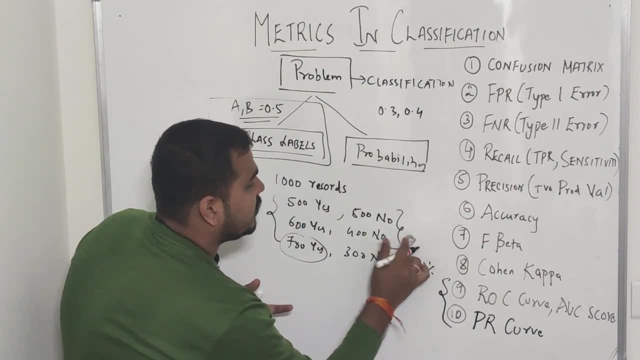 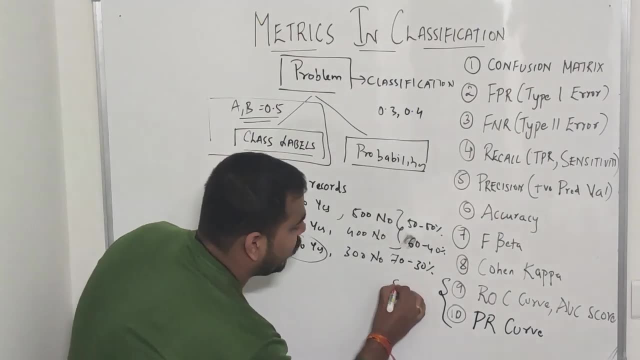 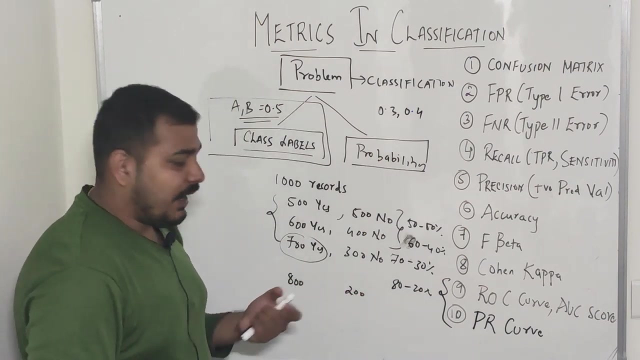 here you have basically like a 60: 40 ratio, here you have 50: 50 ratio, right. but now if i go one more level down, like 80: 20 ratio. 80: 20 ratio basically means that suppose i have over here 800 record and here i have 200, right now in this case. 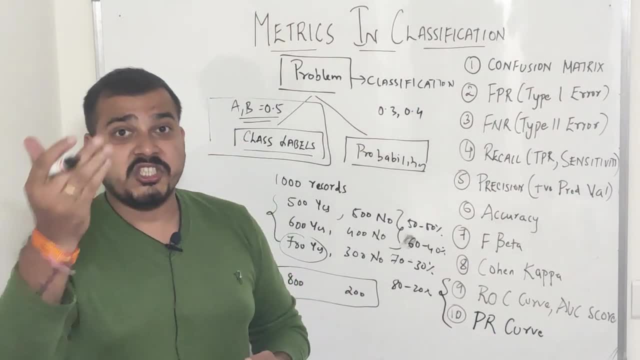 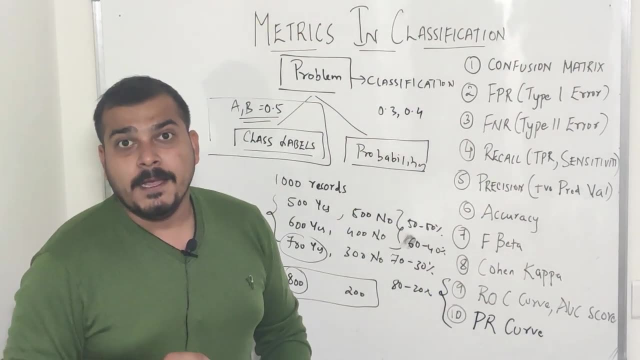 when i provide this kind of imbalanced data set to my machine learning algorithm, some of the machine learning algorithm will get biased based on the maximum number of output. okay, now, if we have a balanced data set, if we have a balanced data set, the type of metrics, that is basically. 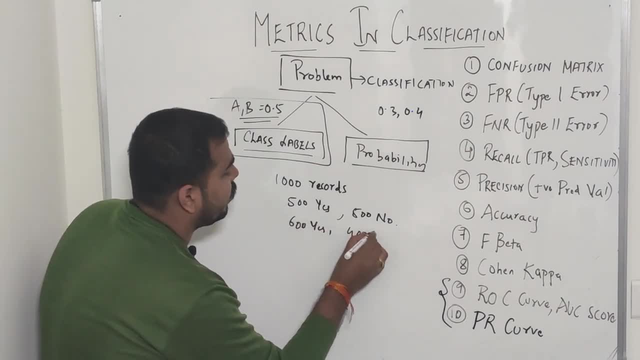 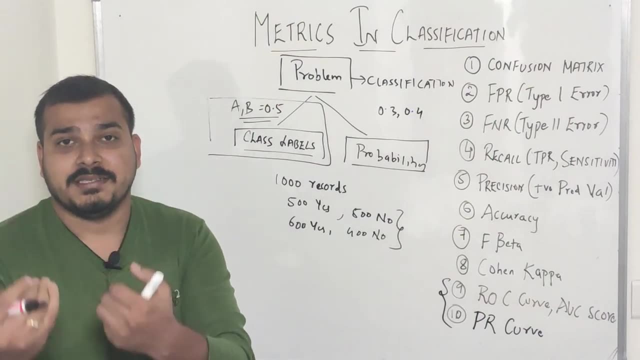 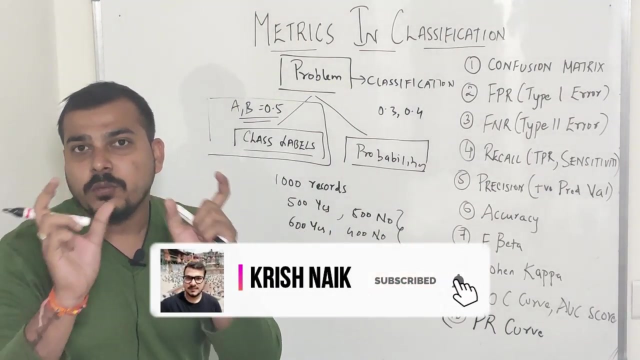 may have 600 years or 400, no, right now. in this case, what I can suggest is that this looks like an M. this looks like a balanced data set. okay, balanced data set basically means that, yes, you have almost same number of years and same number of no, so both the output labels are almost same. 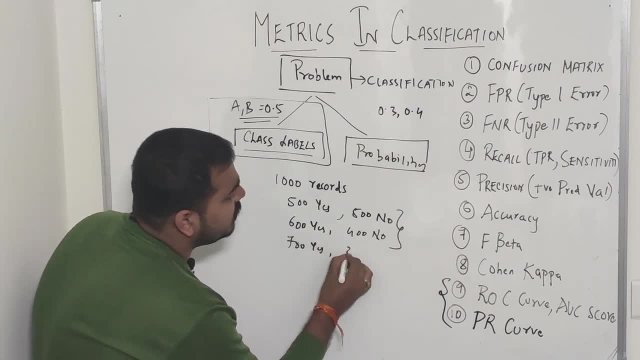 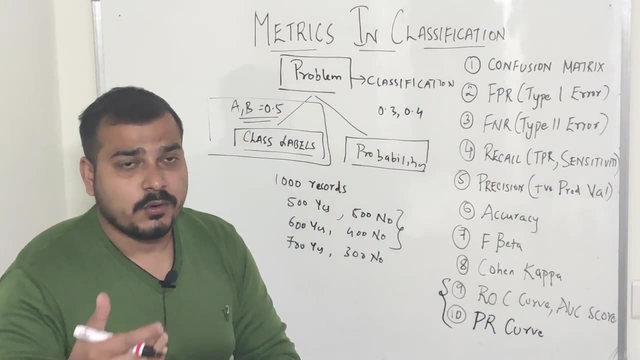 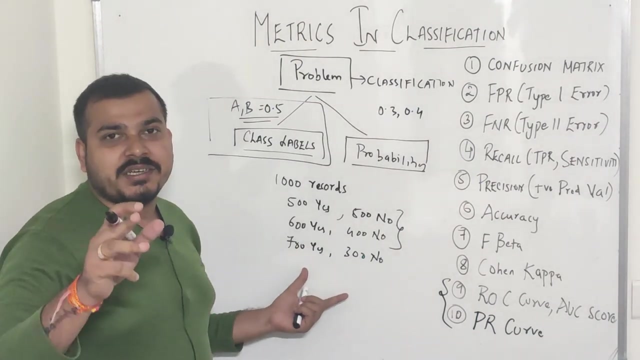 similarly, if you could take 700 yes and 300 no, this is also fine. this looks like a balanced data set. okay, now understand one thing, guys, why? why I'm saying balanced data set? over here, the number of yes and no are almost equal in this case. you may be suggesting, Chris, there is. 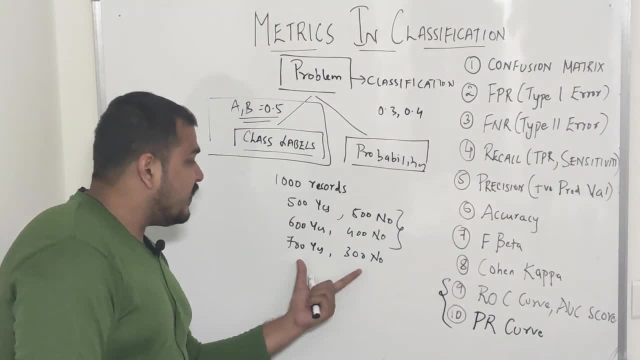 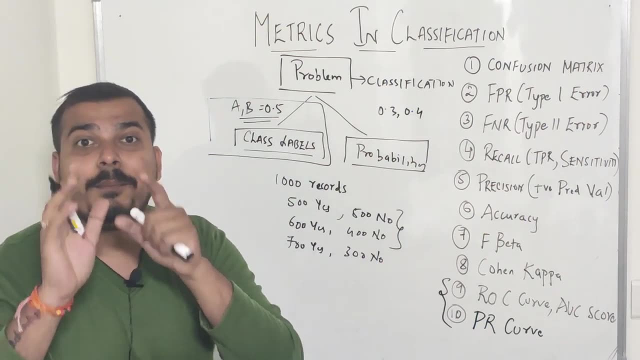 a difference of 400, but it is fine why. I'll tell you if we have this kind of data set also, and if we try to provide this kind of data points to our machine learning algorithm, my machine learning algorithm will not get biased based on the maximum number of output. okay, but if we have scenarios, 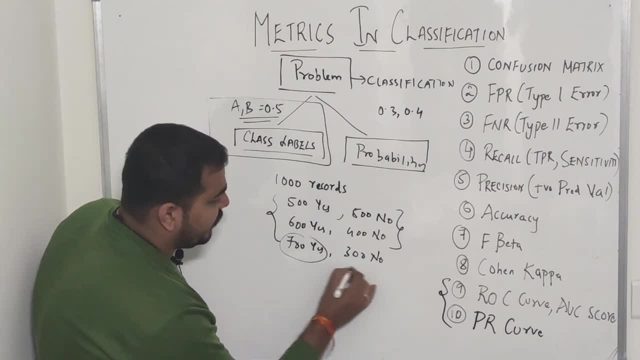 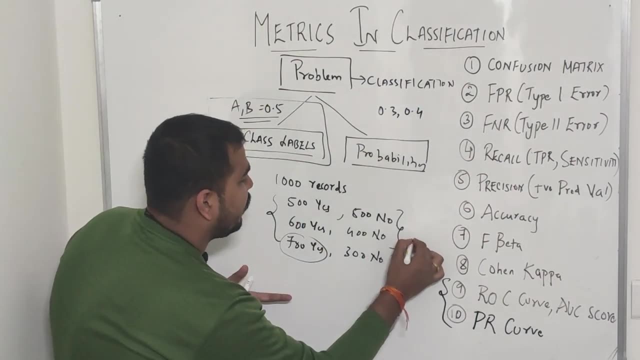 where in our data set ranges- and this is basically 70 to 30 right, 70 to 30 percent- you can see that the number of yes and no are almost equal. in this case you may be suggesting basically 70 to 30 ratio. here you have basically like a 60: 40 ratio. here you have 50: 50 ratio, right. 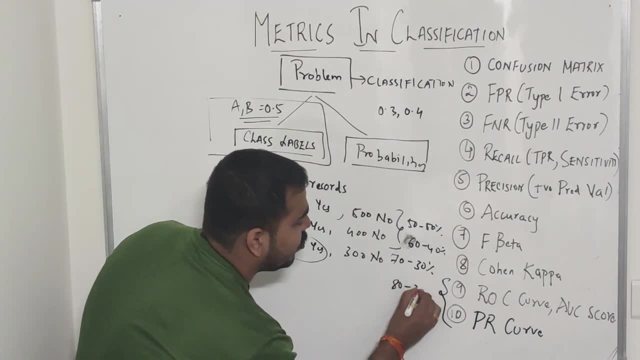 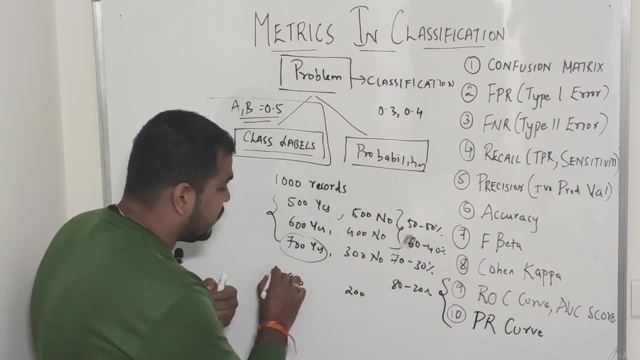 but now if I go one more level down, like 80: 20 ratio, 80 20 ratio basically means that suppose I have over here 800 record and here I have 200. right now, in this case, when I provide this kind of imbalance data set to my machine learning algorithm, some of the machine learning algorithm. 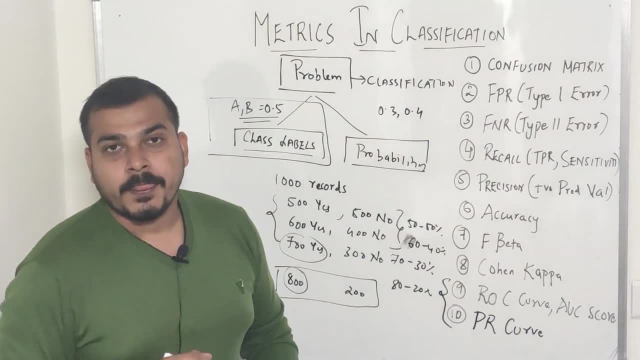 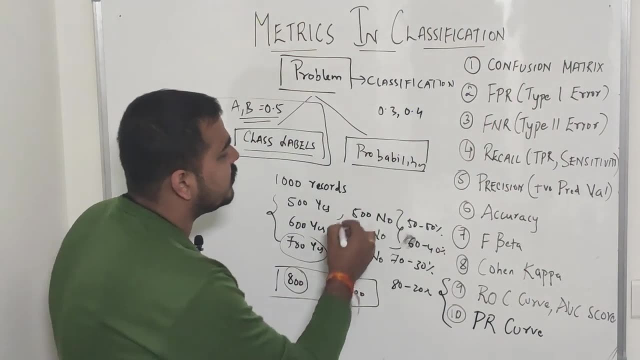 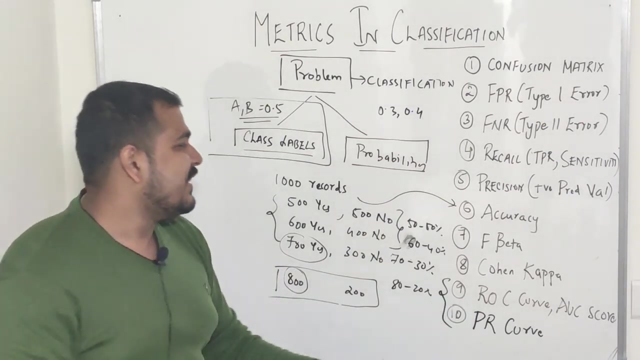 will get biased based on the maximum number of output. okay, now, if we have a balanced data set? if we have a balanced data set, the type of metrics that is basically used is something called as accuracy. if we have an imbalanced data set, at that time we do not consider accuracy. instead, we consider something called as recall, precision and F beta. 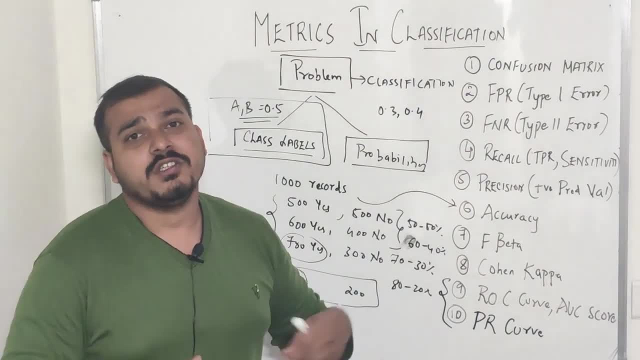 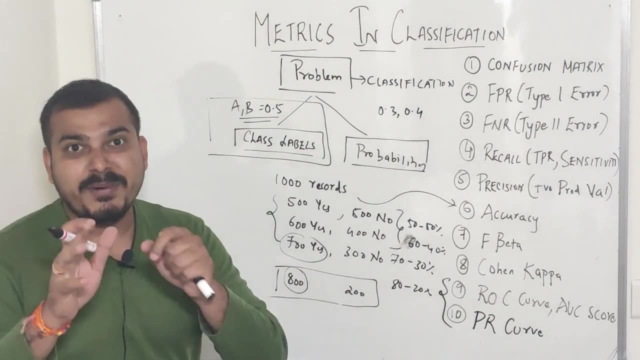 I'll explain you about what exactly is F beta score, which is also called as F1 score, if you have heard of for most of it. but this F1 score is derived by this beta value that will be discussing about now. just consider, guys. initially let us take that, suppose, my data set. 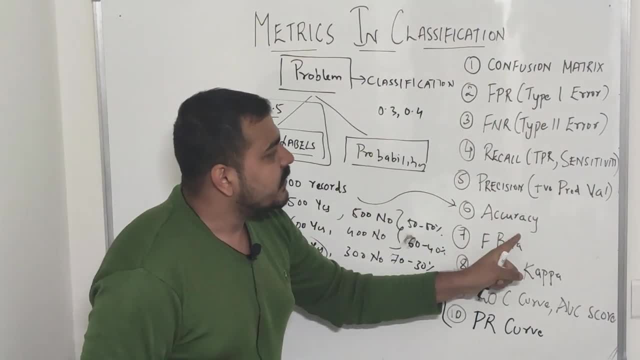 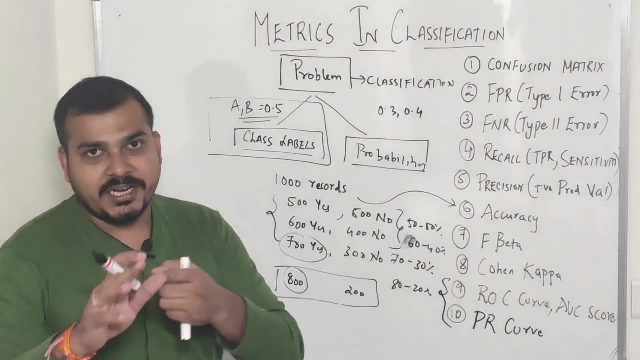 is balanced. okay, at that time I'll try to explain you accuracy and then we will then understand. if our data becomes imbalanced, how do we solve this particular problem? okay, so let us go ahead. I'm just going to rub this thing and if you have not understood, just you know. just go back again, see. 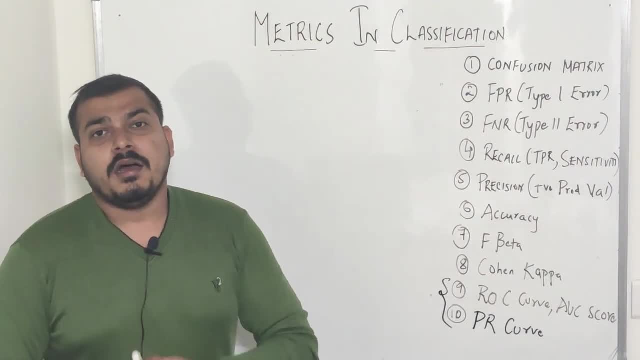 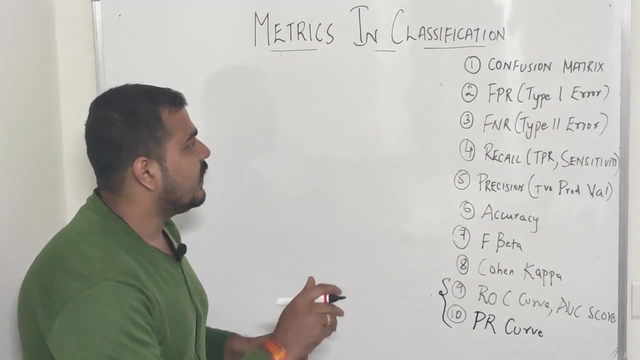 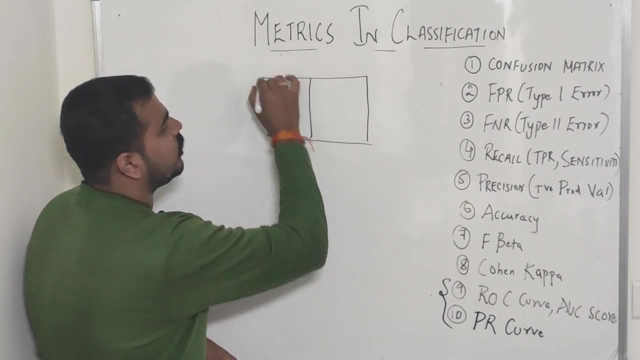 this particular explanation, what I've given. okay, now, first of all, if we have a binary classification problem, guys, we need to understand what is the binary classification problem, guys. we need to understand what exactly is the confusion matrix. now, understand one thing, guys: confusion matrix is nothing, but it is a two cross, two matrix. in case of binary classification problem, where the 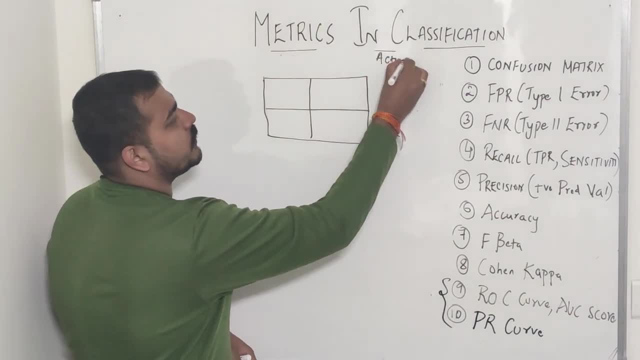 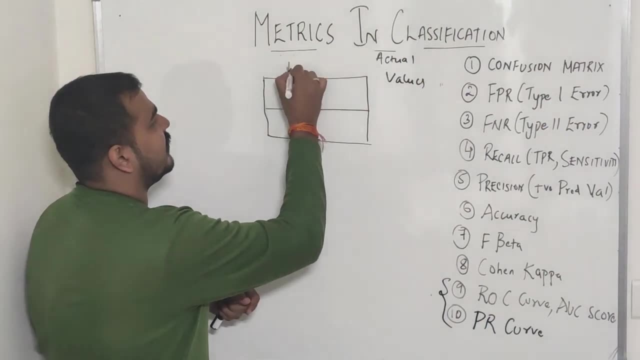 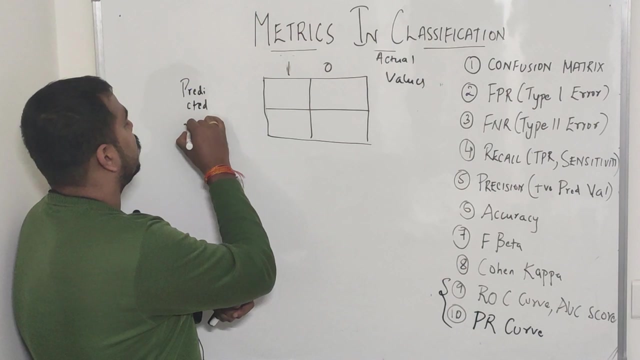 top values are actually the actual values. okay, the top values are the actual values over here, actual values like zero or one, one or zero- suppose I consider this as one and zero- and similarly in the left hand side, this all are my predicted values. so this, basically, values indicate that. 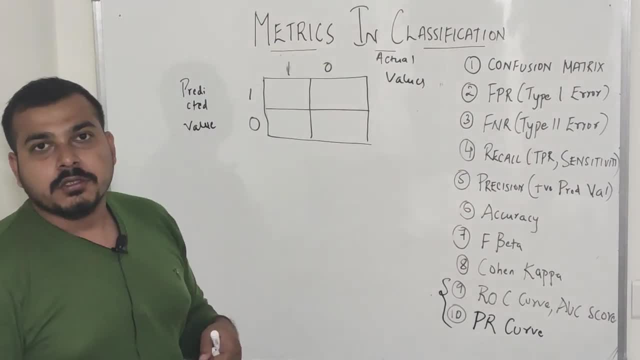 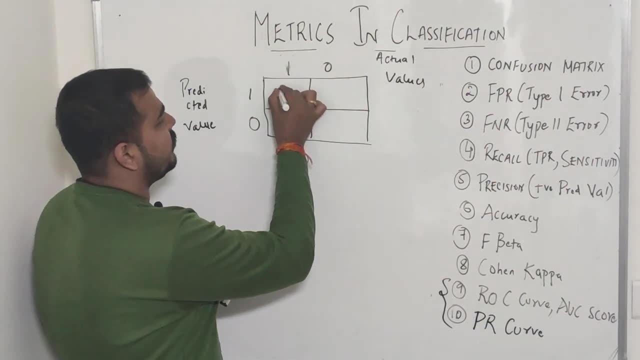 this model has actually predicted, so this will also become one and zero. so usually what we do is that each and every field we specify with some notations. so the first field in this case is something called as true, positive. the second field is something called as true, false, positive and the 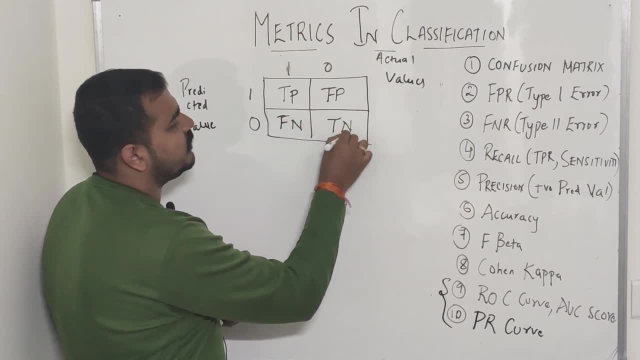 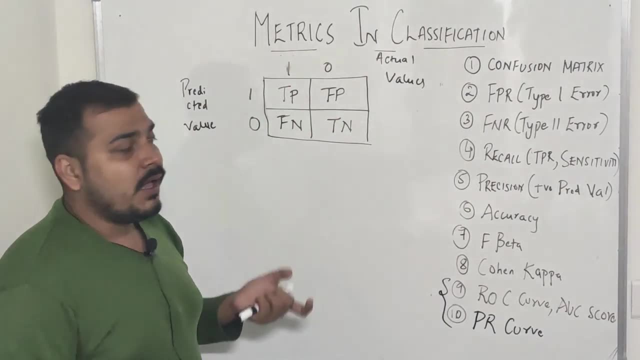 third field is something called as false negative, and the fourth field is something called as true negative. we'll try to understand more in depth what exactly this of these fields mean. okay, what is false positive? what is false negative? and, by default, if I consider this type one, 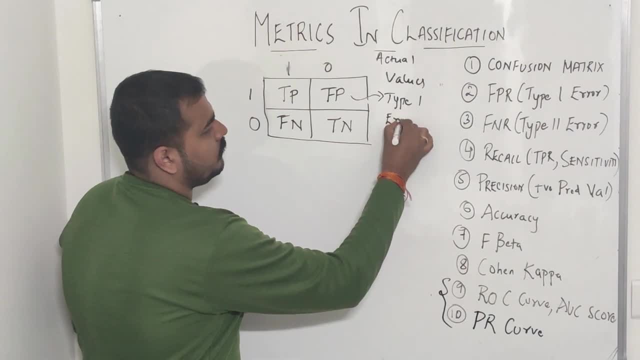 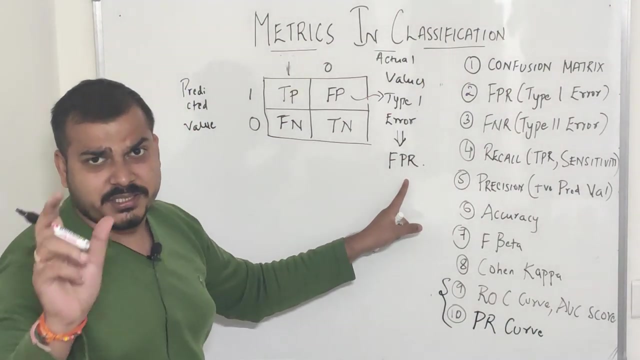 is called as type one error. okay, so if I want to consider this false positive, this is basically called as a type one error. we we can also compute the type one error with the help of false positive rate. okay, false positive rate. I'll define the formula in just a while. this FN is basically. 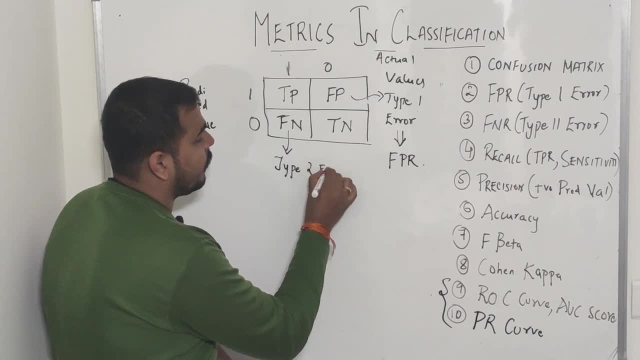 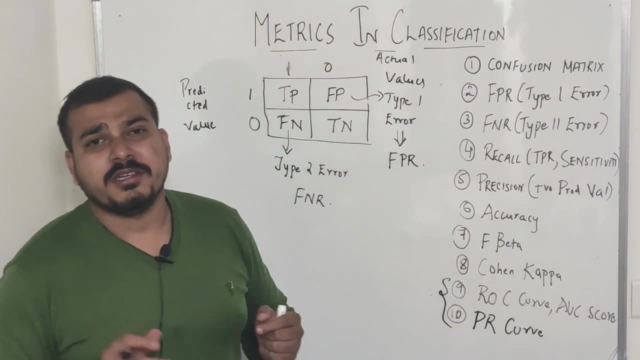 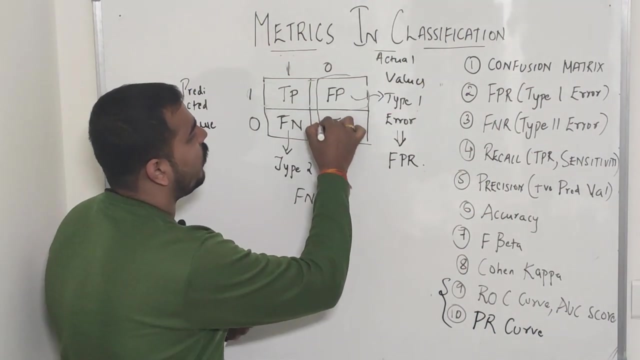 called as a type two error and this is also mentioned like false negative rate. now, what does what? what does this false positive mean? now, if you want to define false positive error, how do we do? is that we basically consider this false values with respect to your actual and predicted and the 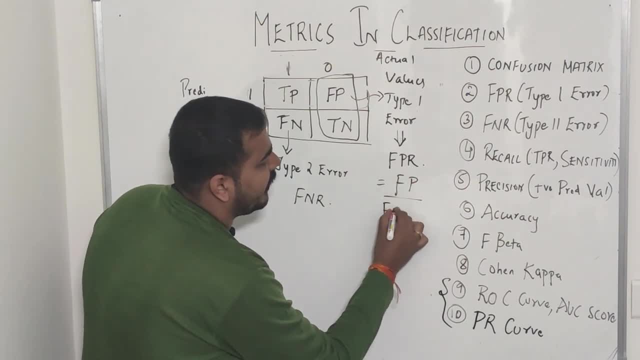 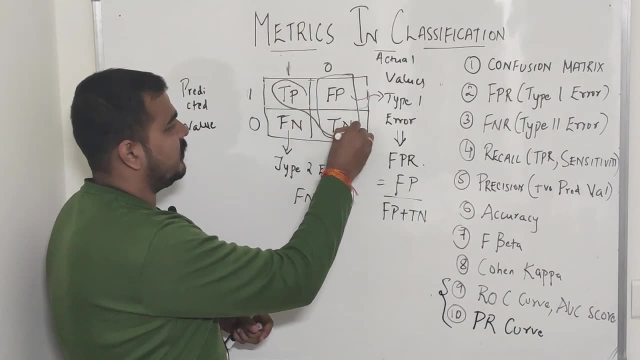 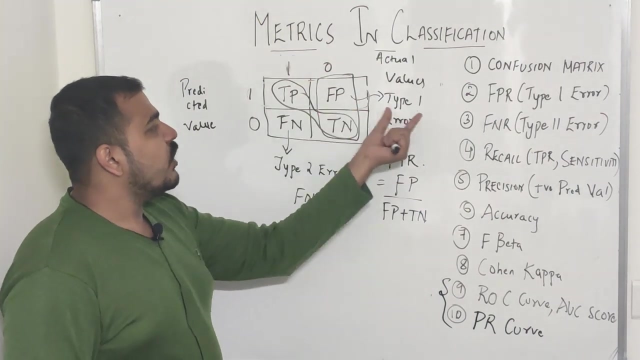 false positive rate is basically given by F P divided by F P plus TN. okay, this true negative and this, and always remember guys, these are your most accurate results. okay, TP and TN. and always your aim should be: okay, in any classification problem, to reduce your type of error. okay, so, 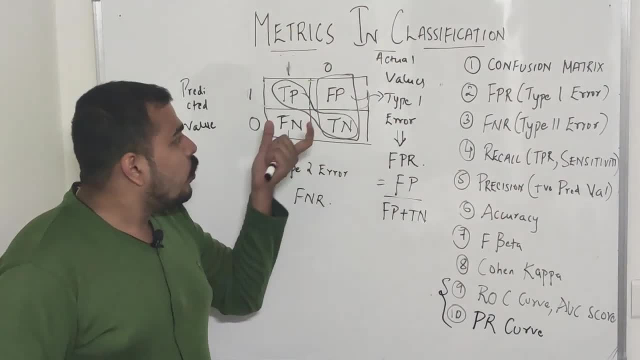 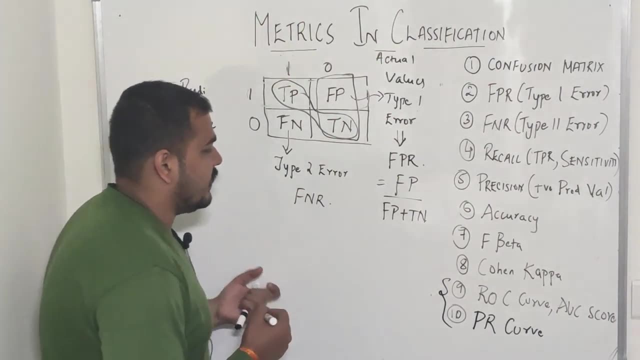 type one error and to reduce your type two error. okay, you always have to focus on reducing your type one error and reducing your type two error. okay, now understand one thing, guys, since this is a balanced problem statement, right, so what we do is that we directly compute the accuracy. now how? 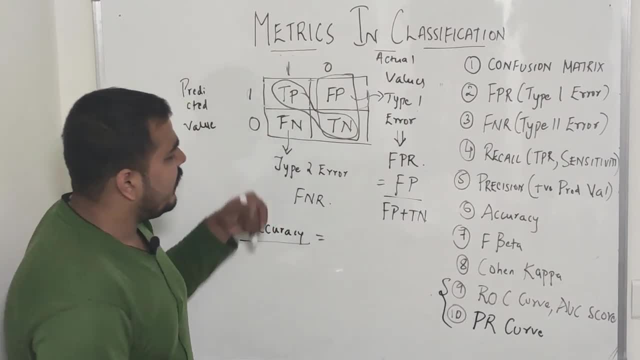 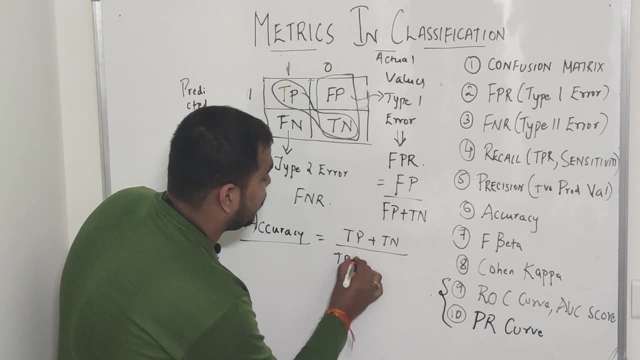 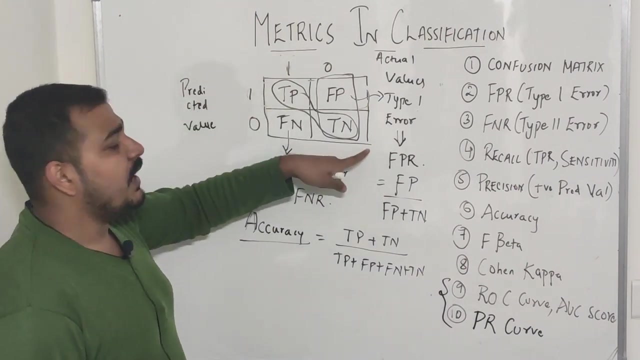 does we? how do we compute? the accuracy is that we simply add TP plus TN, TP plus TN divided by TP plus FN, fp plus fn plus tn. that basically means i'm just saying that this diagonal elements, which will actually be giving me the right result, divided by total number of elements, and this will give 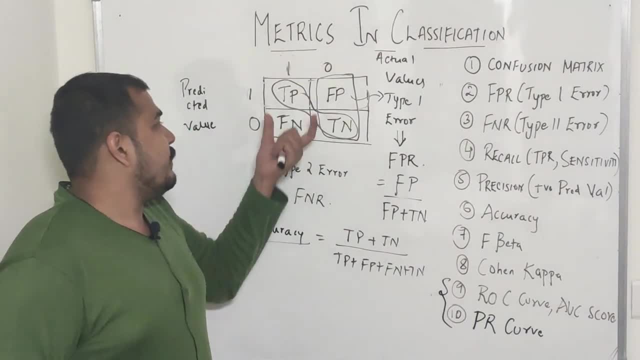 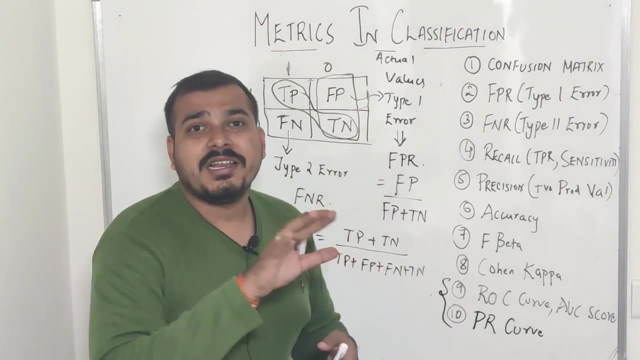 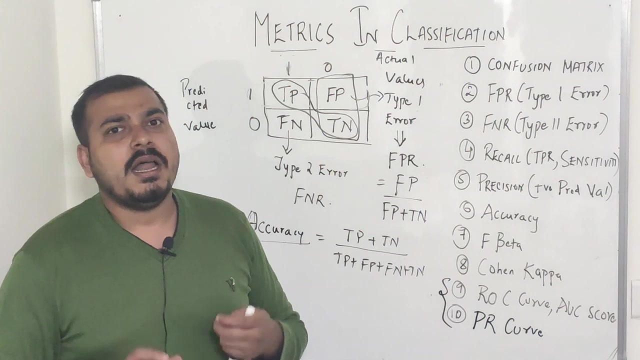 us the accuracy why i'm following this particular stuff, because i'm considering this problem statement is my balanced data set? okay, and during the balanced data set, usually my model does not get biased based on the different types of categories that we have in this binary classification problem. okay, but now what if? what if my data set is not balanced? what if my data set is not? 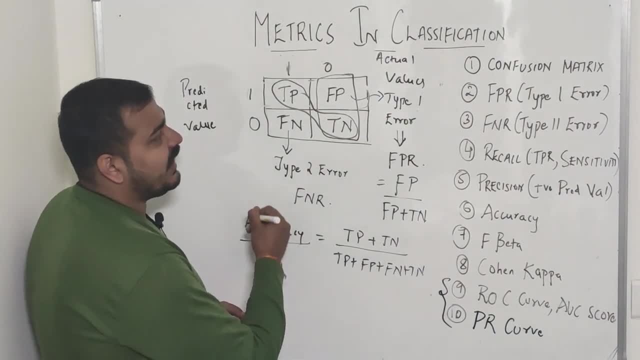 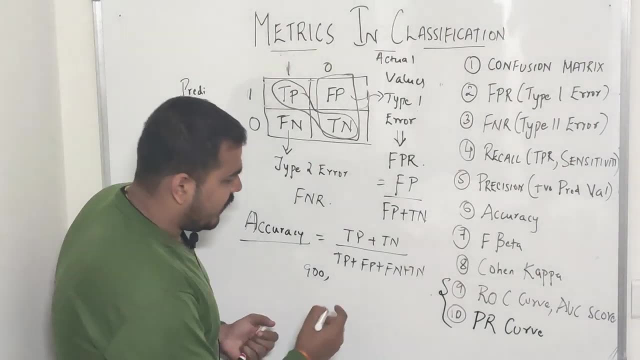 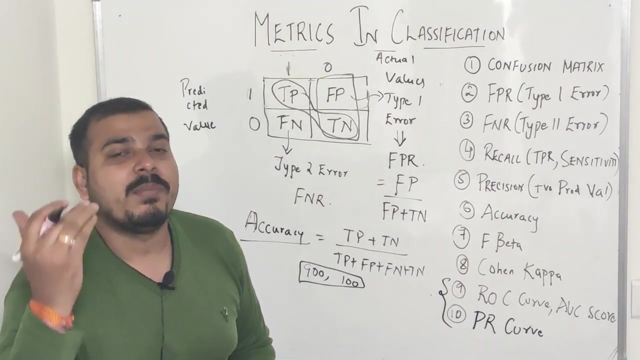 balanced. let me give you a very good example. suppose one category, one category, i have some hundred, nine hundred values. suppose out of the thousand records i have nine hundred, one category and hundred as my another category, okay, hundred as my another category. now, if i apply, just understand over here, guys, if i just say that my model will blend. 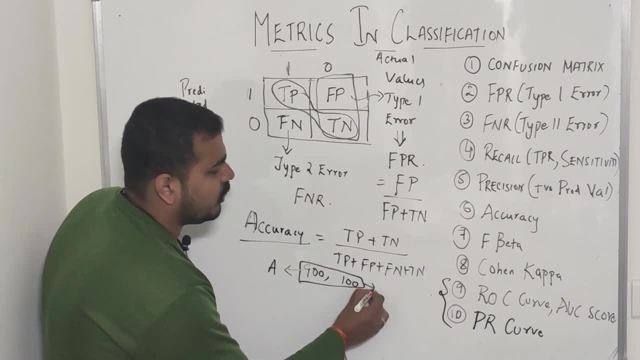 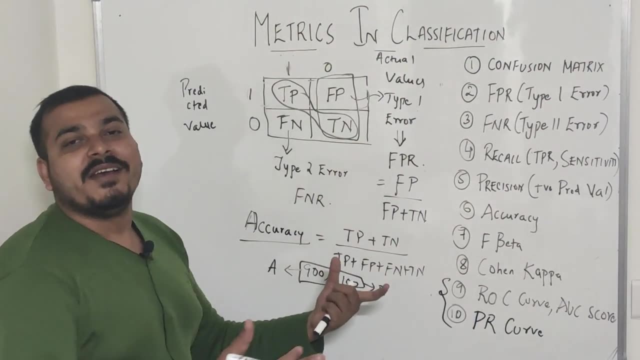 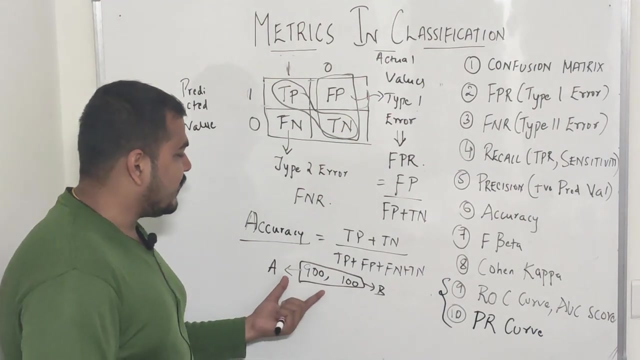 i will say that everything belongs to category a and not to category b. okay, not to category b, but instead it will say that every, every- i mean every values or every test data set belongs to my category a instead of category b. okay, so out of this, i'm just suggesting that. okay, nine hundred. 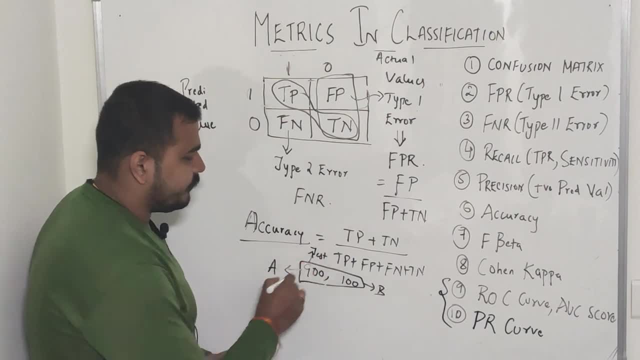 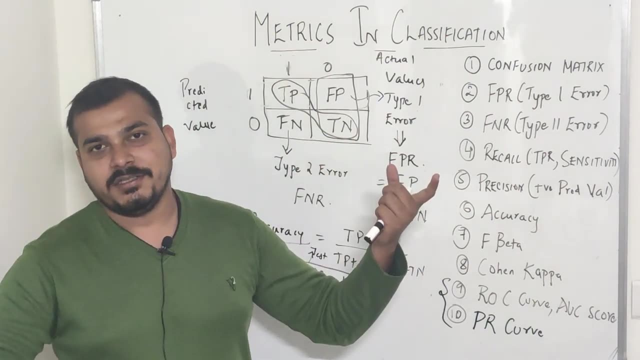 values and i'm considering this is my test data. suppose, guys, okay, suppose i'm having this test data. or just consider that i had my trained data. in my trained data, i had, uh, fifteen hundred records, out of which twelve hundred was my uh- a classic category uh- and three hundred was my class b. 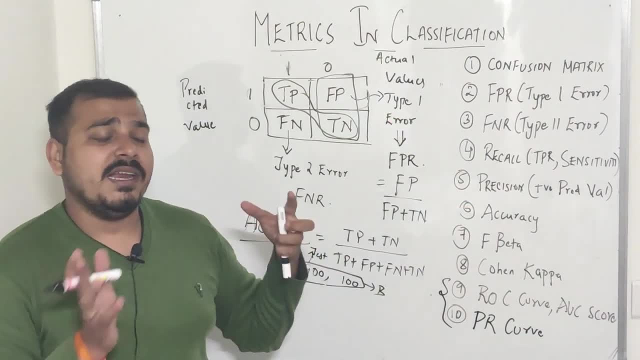 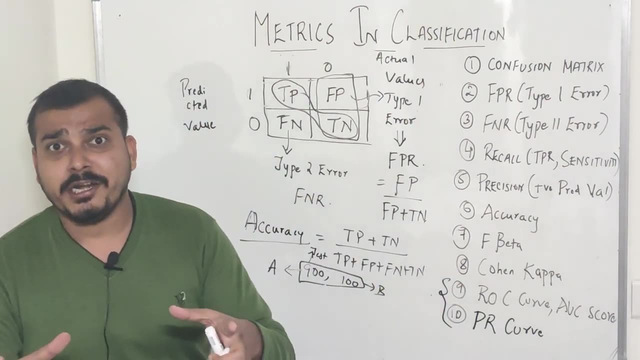 category and now i have divided that into train test split my in my inside my test data. suppose i had around. uh, i'm just considering an example. in my test data i had class a as nine hundred records and class b as 100 records. now suppose if my model predicted all the classes were class a. 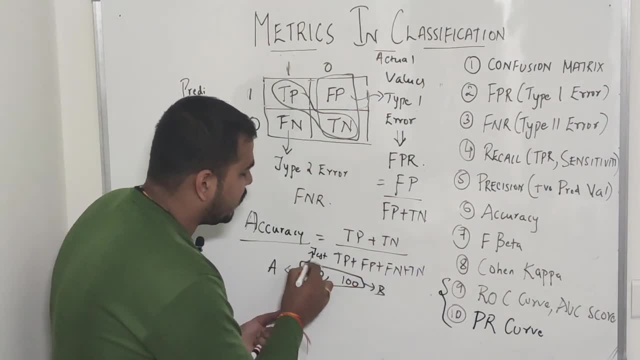 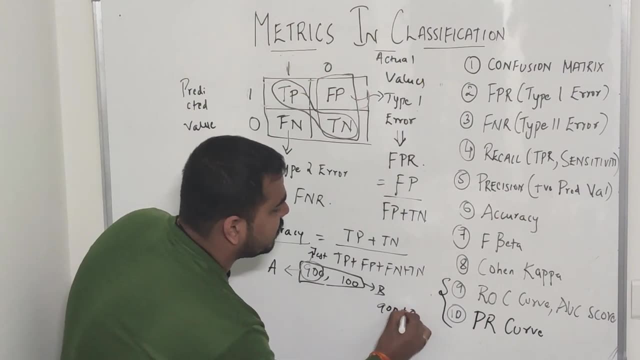 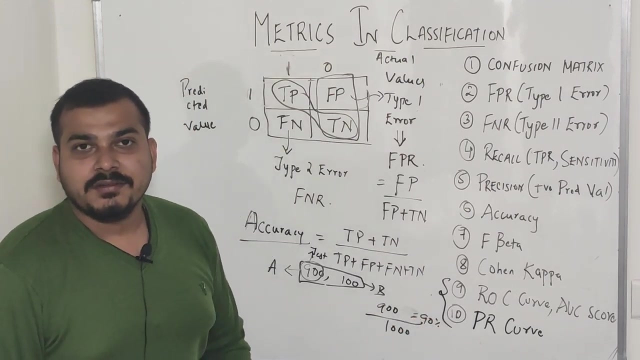 now, in that specific case, if i said tp plus tn, i'm just going to get the 90 accuracy right, because positive i'll be getting 900, true, negative i'll be getting zero, and if i do the submission of all of this, this will become thousand. and this is, in short, 90 percent of accuracy right. so this is a. 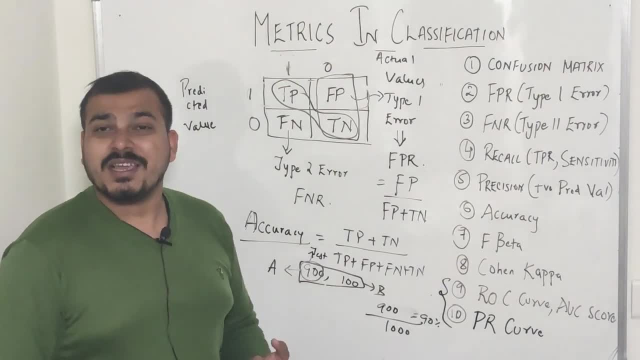 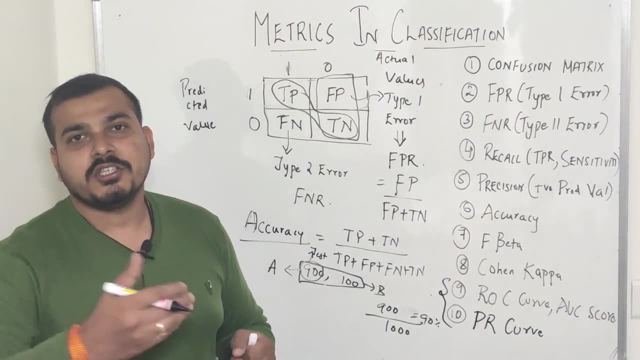 problem, right. if we have an imbalanced data set, we cannot just use accuracy, because it will give you a very, very bad meaning about that particular model. you know you're just blindly saying that it belongs to just one category. so if you have an imbalanced data set, you basically go with. 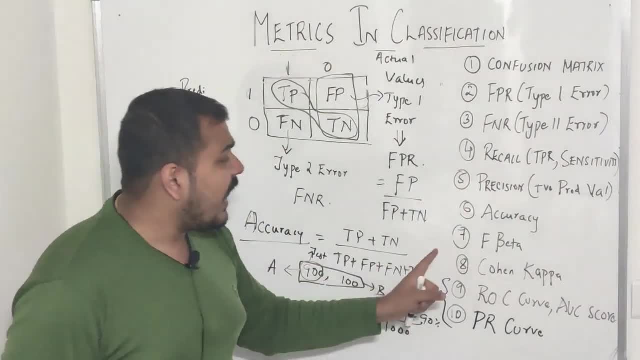 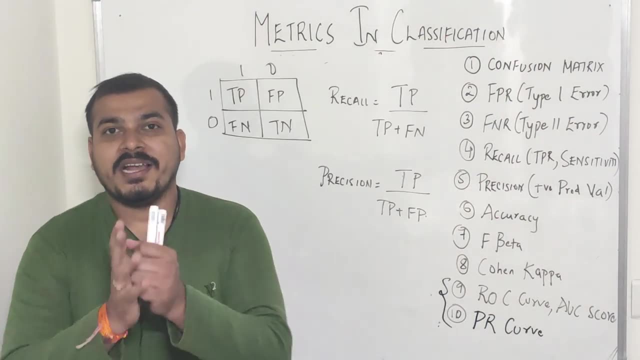 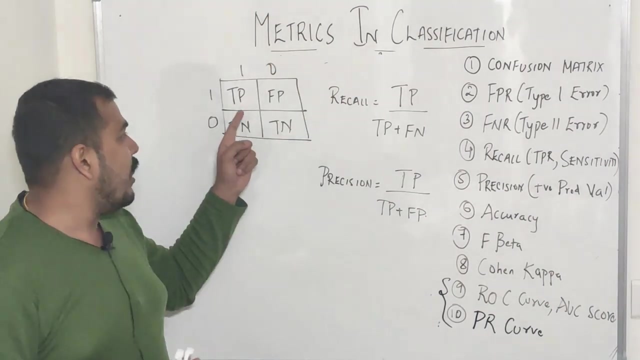 something called as recall, precision right, and something called as f beta score. now let us go ahead and try to understand about recall and precision. okay, guys, now let us go ahead and just understand what exactly is recall and precision? now, guys, here is my confusion. matrix: here you have true, positive. 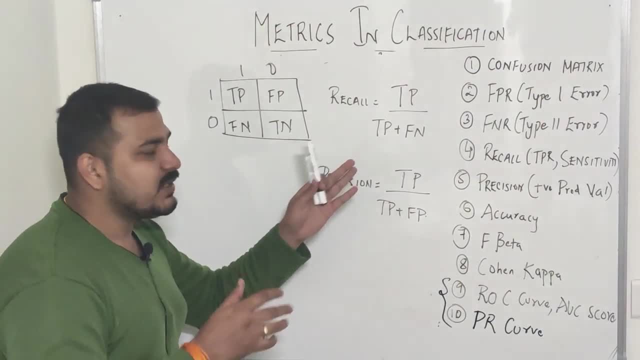 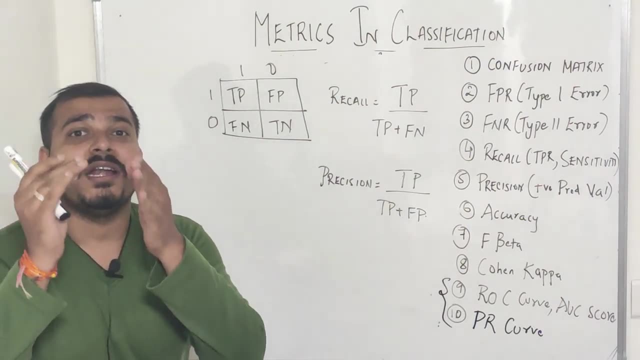 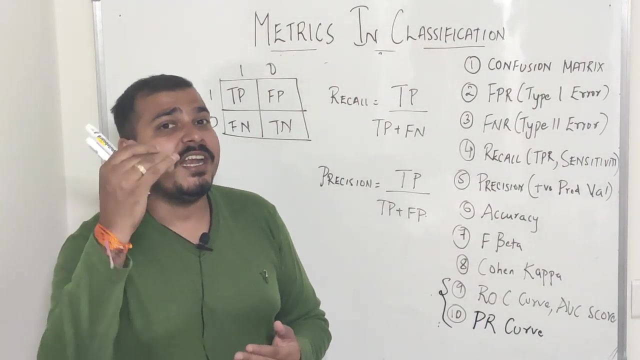 false positive, false negative and true negative. understand why do we use this for an imbalanced data set? now understand one thing, guys: any kind of data set that you have, you should always try to reduce your type one error and type two error. okay, you should always try to reduce this. Now, specifically, when your data set is: 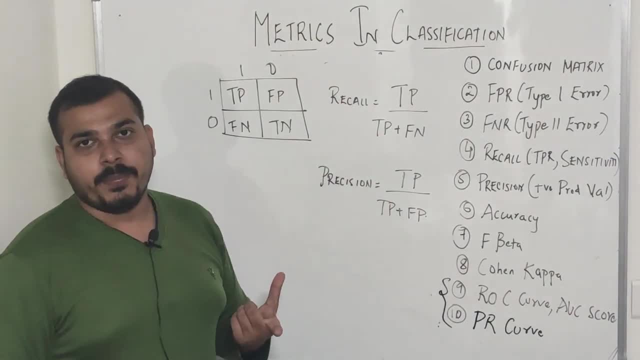 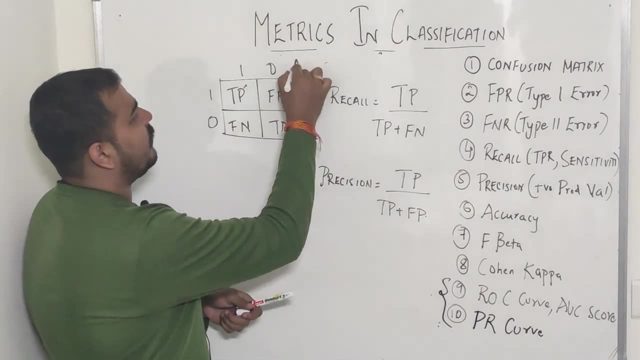 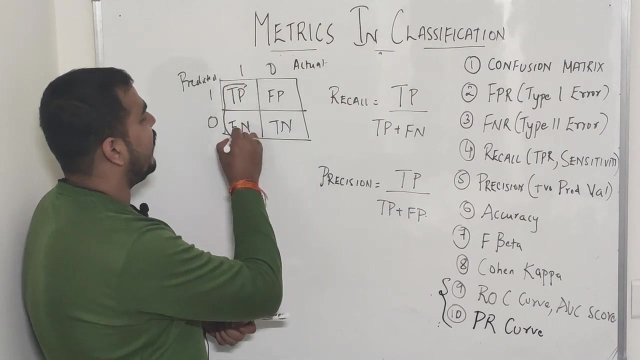 imbalanced. we should either focus on recall and precision. Now, what does recall over here formula says? Recall basically says that TP. so these are my actual values, right, these are my actual, these are my predicted values. so this basically says that TP divided by TP plus FN- okay, TP divided by TP plus FN. 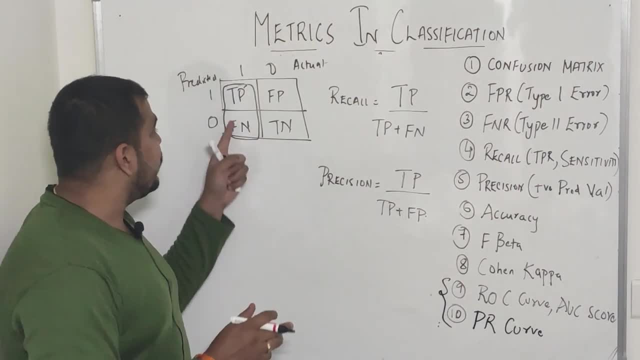 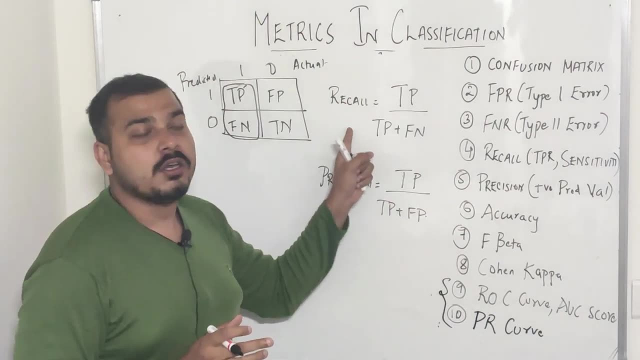 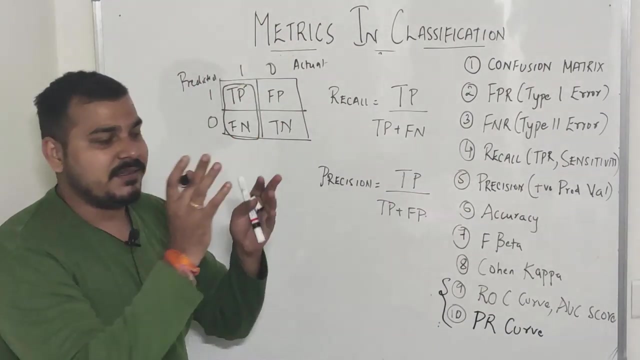 now, what does this? says that, out of the total positive actual values, how many values did we correctly predicted? positively? okay, this is what this recall basically says. again, I am repeating it, guys: out of the total actual positive values, one is positive. right, I can say true or positive, anything out of all. 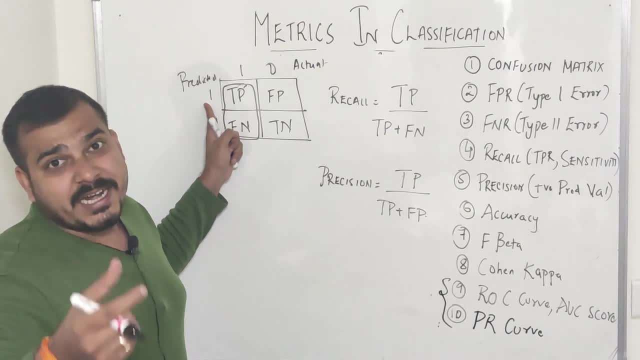 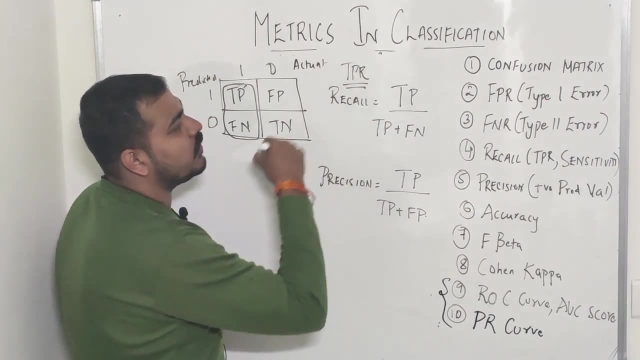 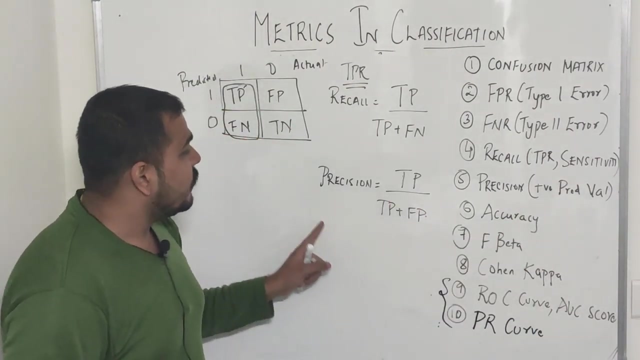 this. how many positive did we predict correctly? that is what this recall basically says. recall is also given by something called as true positive rate. it is also mentioned by to positive rate, or it is also mentioned by sensitivity. okay, it is also mentioned by sensitivity. now, similarly, if I consider 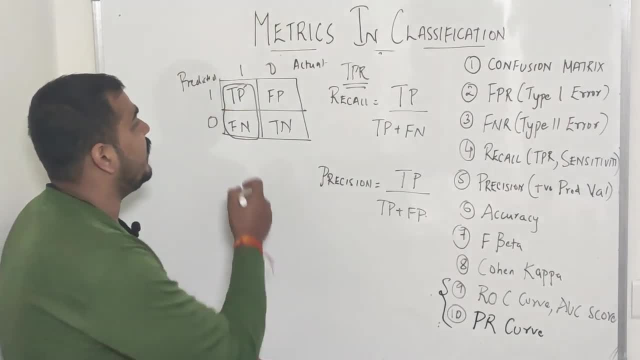 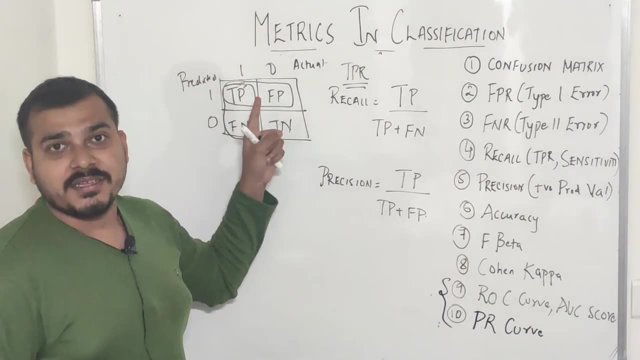 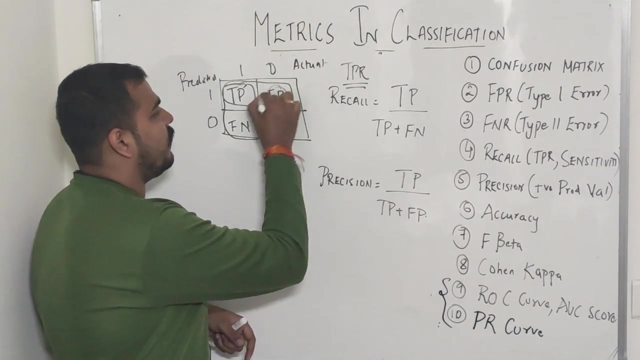 about precision. it basically says: TP divided by TP plus FB. okay, now, what does this basically say? out of the total predicted positive result, how many results were actual positives? okay, here we are actually focusing on the false positive. here in the recall, we were actually focusing on false negatives. 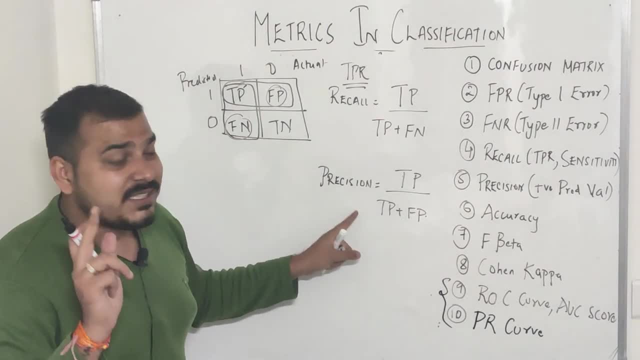 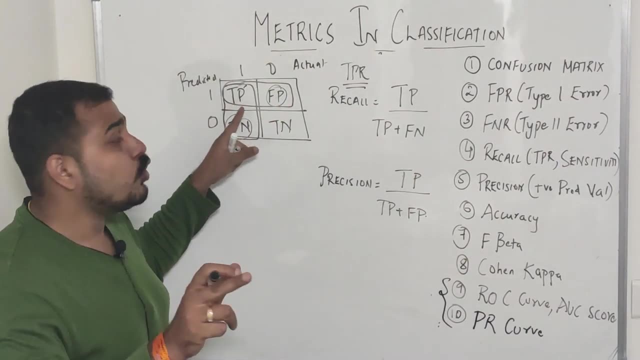 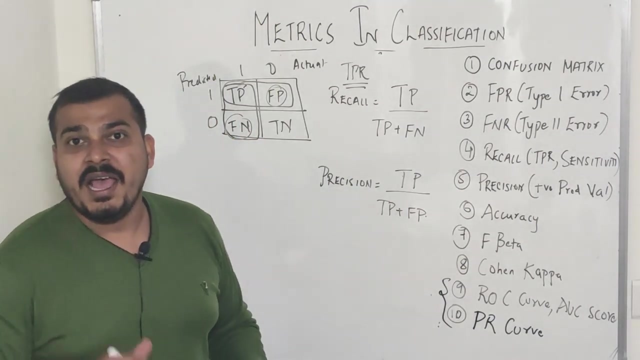 right. so again I'm repeating it: what does precision basically say? out of the total actual positive predicted results, how many were actually positive and what is the proportion that were actual positive? that is what this particular precision basically say. and for precision we also specify another name which is called as positive prediction value. suppose in your interview they 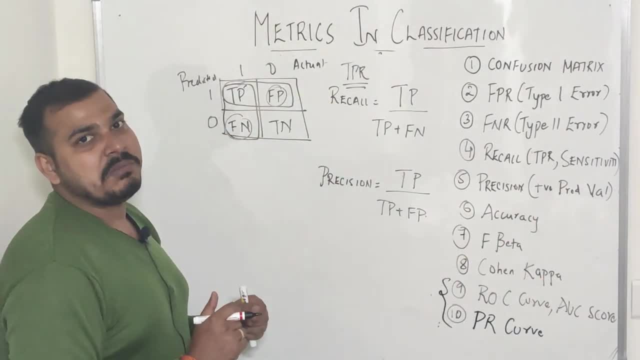 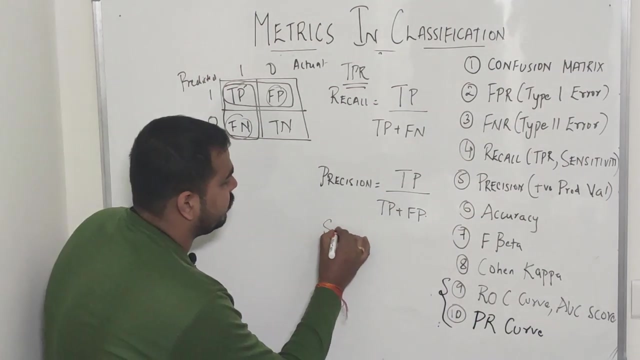 ask you what is actually positive prediction value? you have to explain the same thing. understand this thing, guys. now when should we use a recall and precision? understand, guys? let me just give you some very good example of recall and precision. so I have a use case which is called as spam detection. 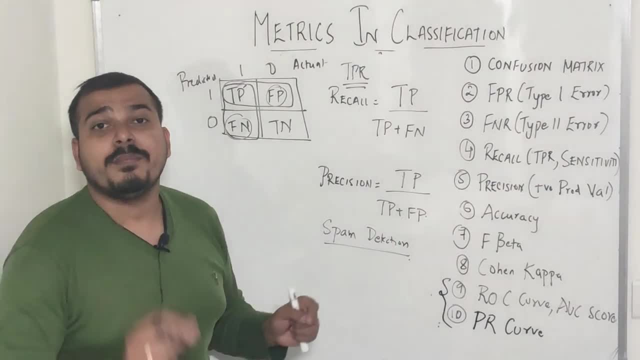 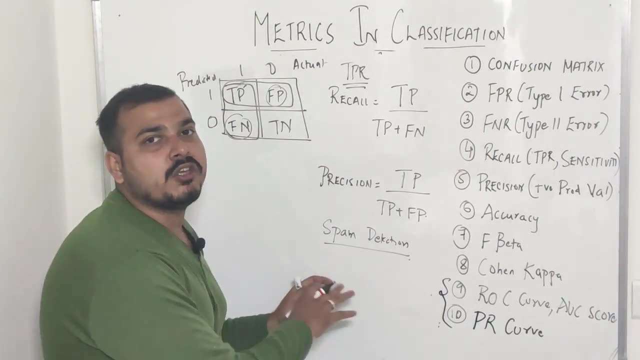 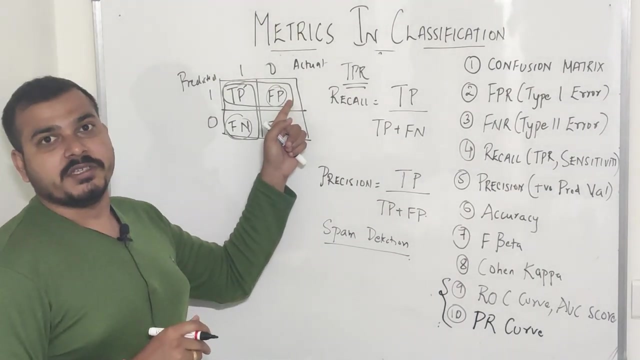 in spam detection I have to focus on precision. why consider that? suppose in this false positive which basically says that: suppose this, this mail is not a spam. okay, suppose it is, mail is not a spam, but the model has predicted that it is a spam. that is your false positive. okay, again, I'm telling you guys, the mail is not a. 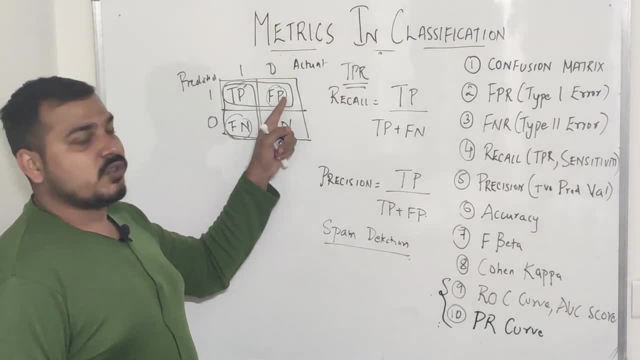 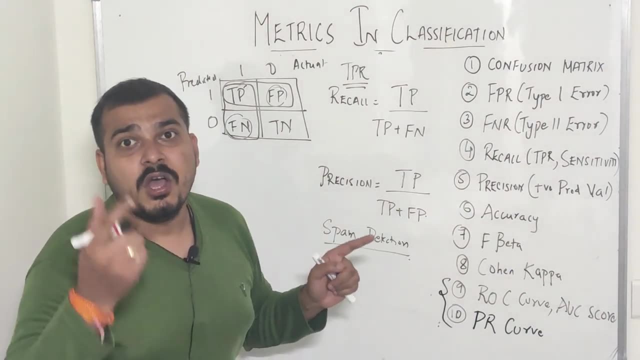 spam, but it has been predicted that it is a spam. so this is what it is saying: zero basically means not a spam, but it has predicted that it is a spam. now, in this particular scenario, what will happen is that we should try to reduce this false positive value. we should try to reduce it: false positive value. 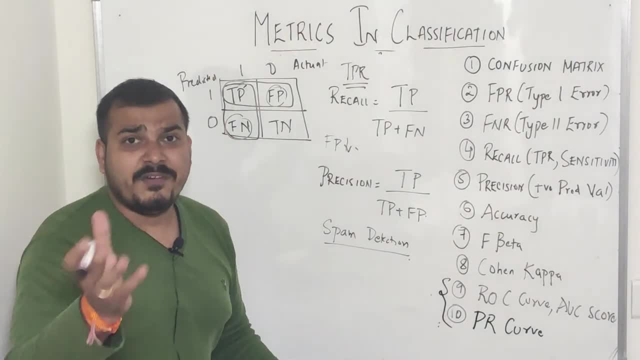 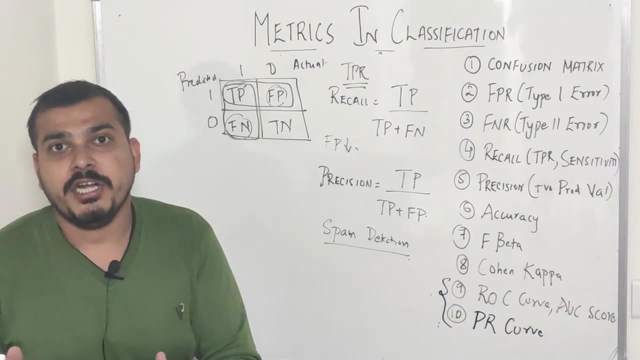 because, understand, in this case, in a spam mail detection, if it is not a spam and if it is specified or predicted as a spam, the customer is going to miss that particular mail, which may be a very important mail itself, right? so because of that we should always try to reduce this false positive value. in the case of 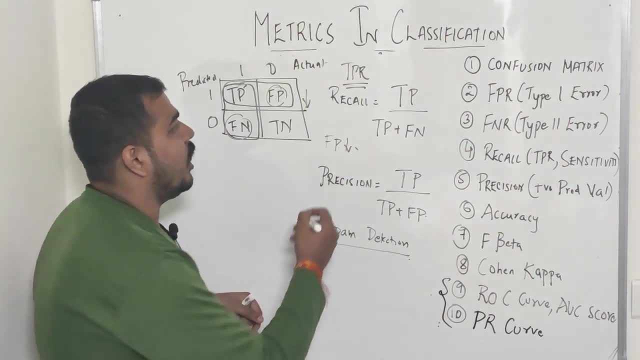 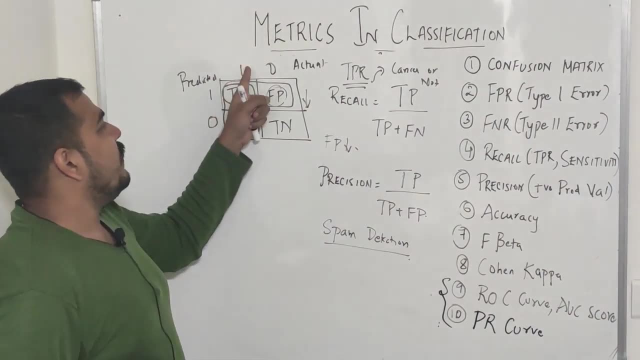 this kind of use case, that is, spam detection. but what about recall? suppose I say that whether the person is having cancer or not, cancer or not, okay, so my one value basically specifies that he is having cancer, zero specifies that he's not having cancer. now, in this particular case, we should. 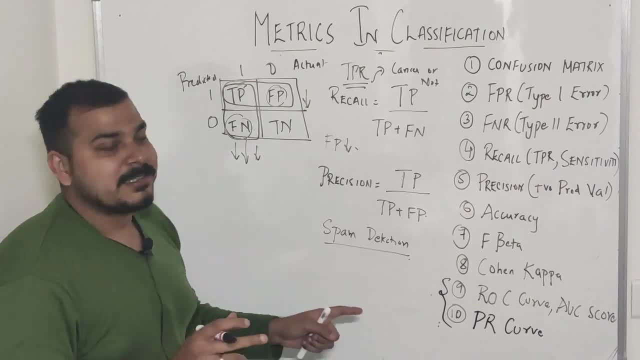 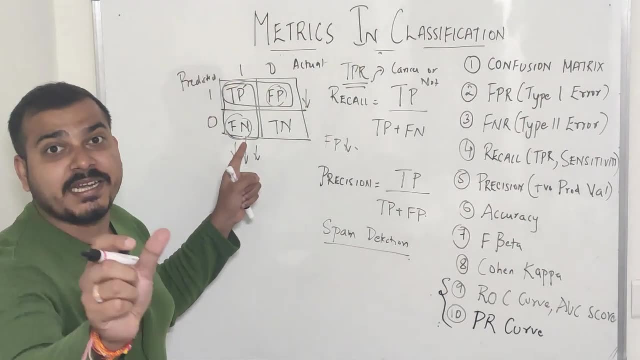 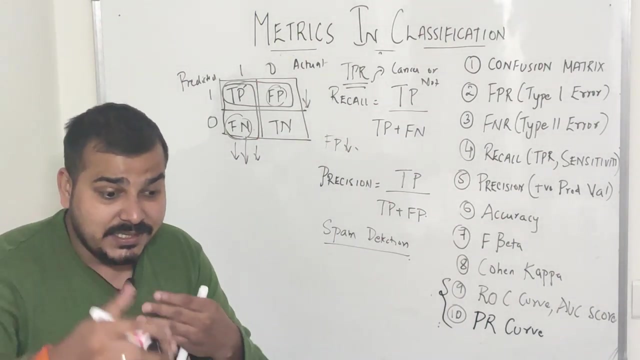 try to reduce false negative. why understand this, guys? this one: now consider that if the person is having a cancer, actually is having a cancer, but he is predicted as that the person is not having by the model. okay, so that is what says over. here is our actual value? suppose is he is suffering from cancer. 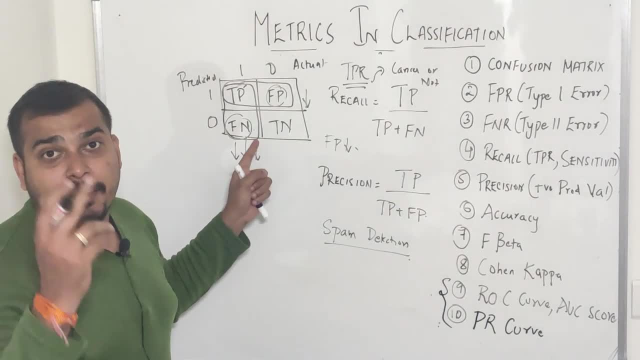 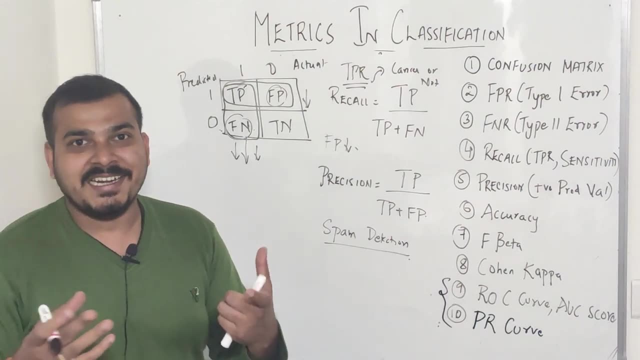 so that what? what exactly the actual value says: right, but the model has predicted that the person is not having a cancer, so this may be a disaster because, again, understand, it is a personal, available model. okay, if you see this person has cancer in患了患病的家庭. 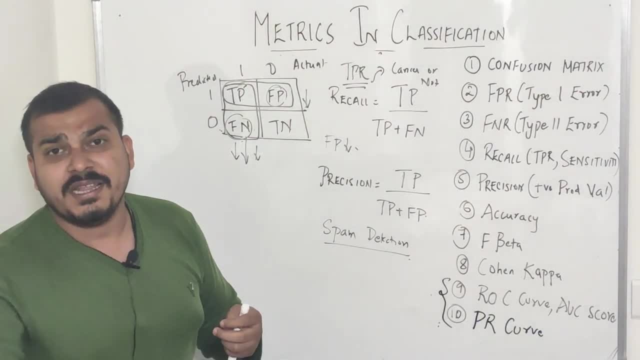 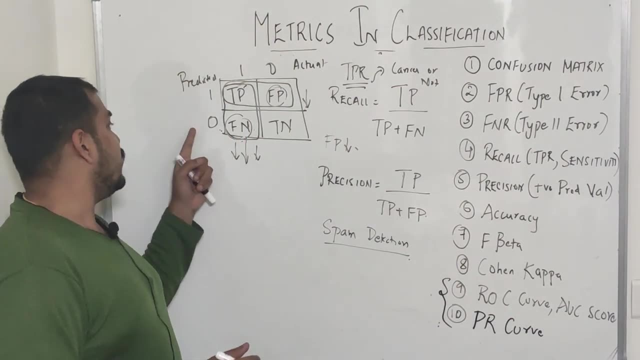 if I get an error in false positive, then the person will go with another further test to understand whether he is having cancer or not. but if my model predicted that even though he had a cancer but he has, so he was predicted as he was not having a cancer, so this is a disaster, at that time we should specifically use 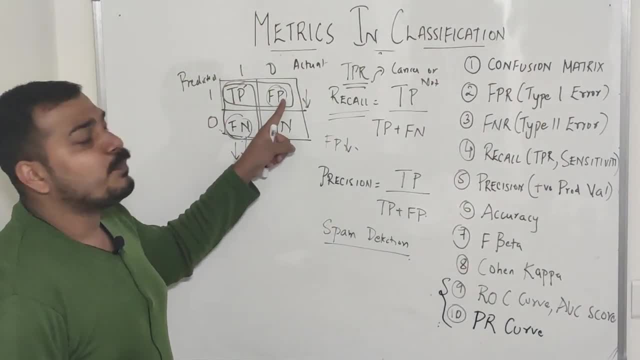 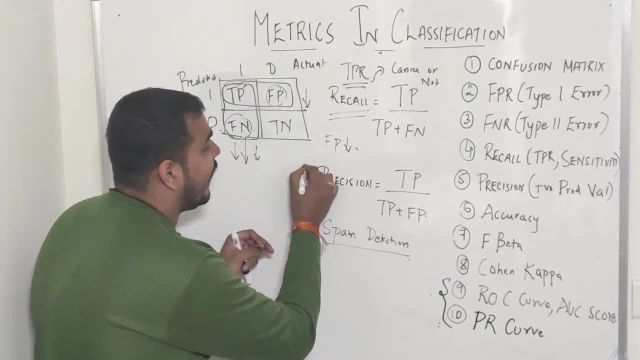 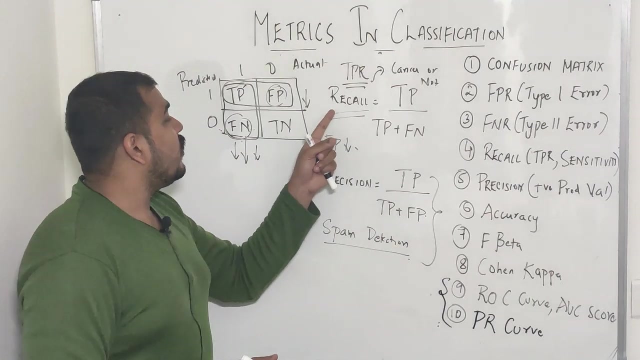 recall now. in short guys, whenever your false positive is much more important, whenever your false positive is much more important, go and blindly use precision whenever with respect to your problem statement. if your recall, if your false negative is important, at that time you go and use recall. I give you an. 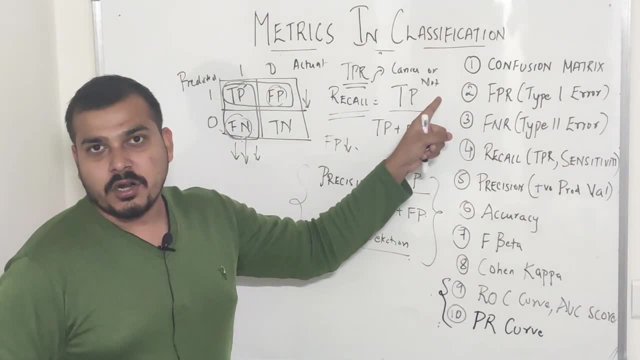 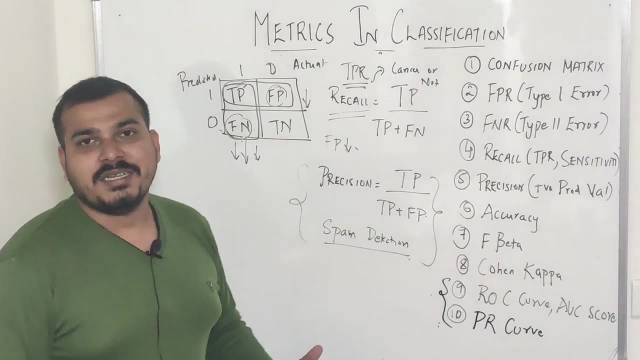 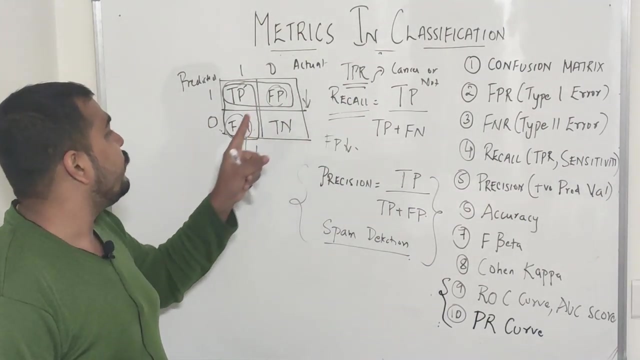 example guys. okay, cancer, whether a person is having cancer or not. some more examples whether tomorrow the stock market is going to crash or not. some example of precision spam detection. right, consider this particular example. try to think. always. our aim should be to reduce false positive and false negative, but whether false positive is playing a 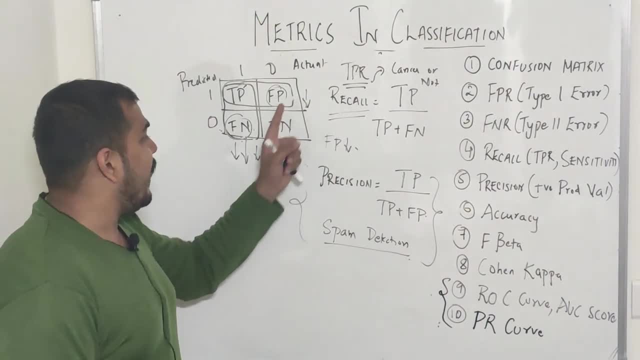 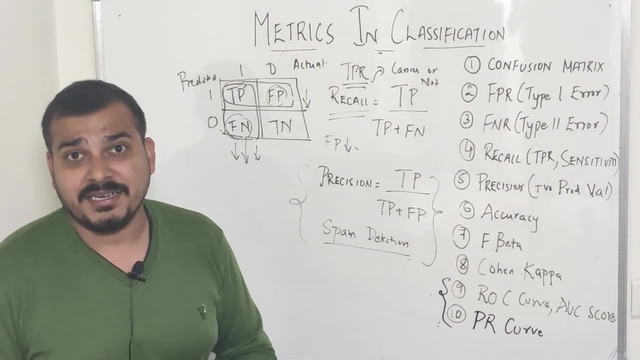 greater impact or role in that specific model. if it is playing, go and use precision. focus on precision. if false, negative is actually playing a greater role or a greater impact it is having, just go and use recall. now I want to introduce you to something called as F beta. now, sometimes, in some of the 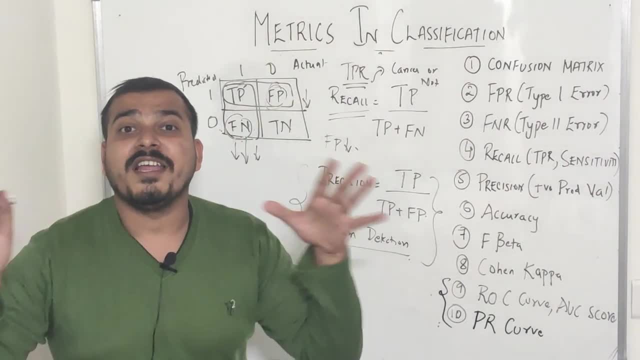 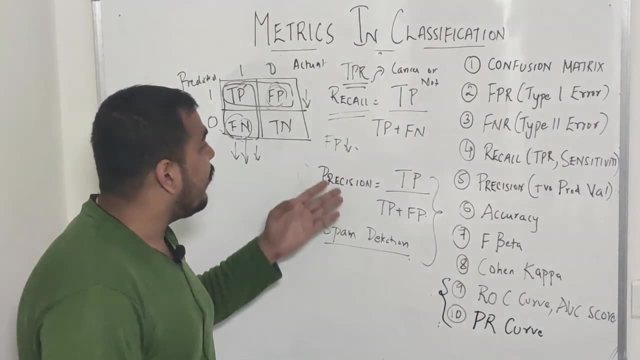 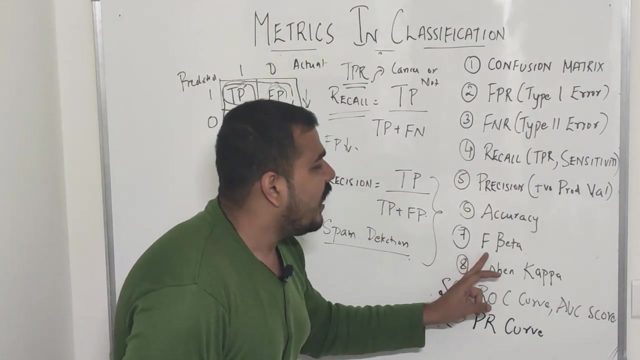 problem statement guys: false positive and false negative. both are very, very important. okay, in an imbalance data set, I'm saying, okay, both will be important. at that time we have to consider both recall and precision. and if you want to consider both recall and precision, we basically use F beta score. okay, F beta score. and sometimes in some of the problem, 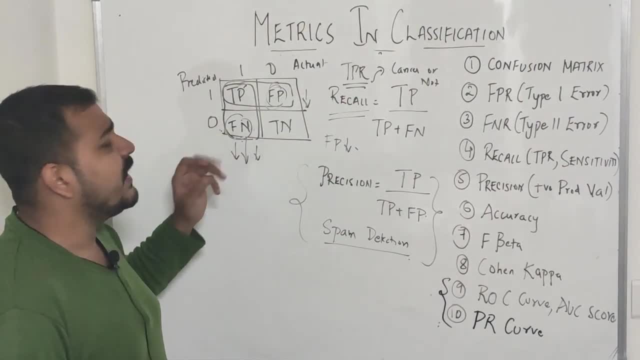 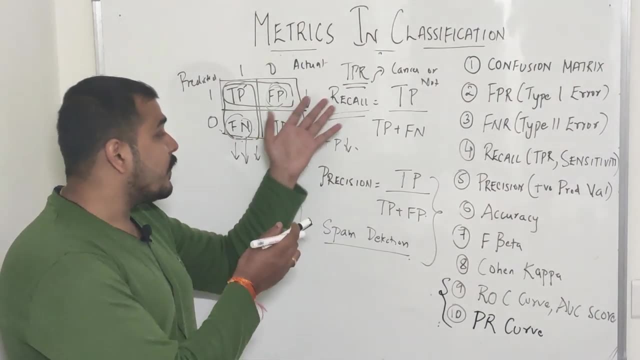 statements, guys, even though recall play a major role, that is like false negative player is major role or a false positive play a major role. you know some of the problem statement. you should try to combine both precision and recall to get the most accurate value. so for that reason I am going to show you the problem statement. 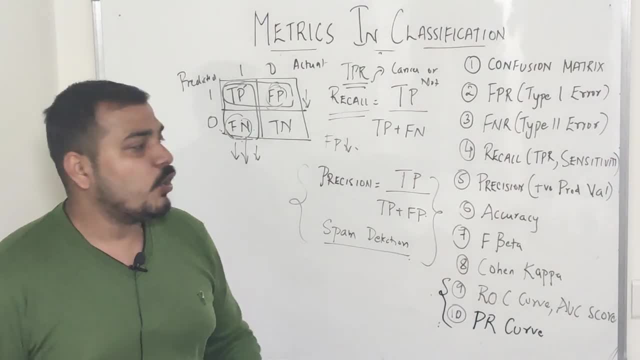 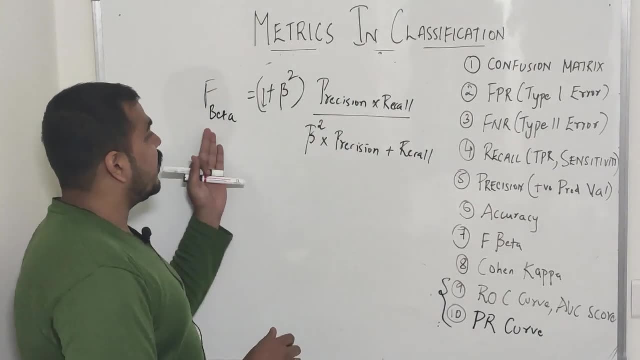 that particular case, we use a F beta score. Now here I'm going to define a F beta score formula for you so that you'll be able to understand. So now let us go and understand. what exactly is the F beta score? guys, In F beta, usually the main aim is to select this beta value. 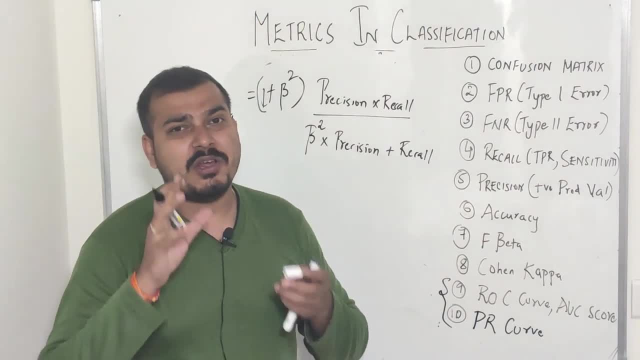 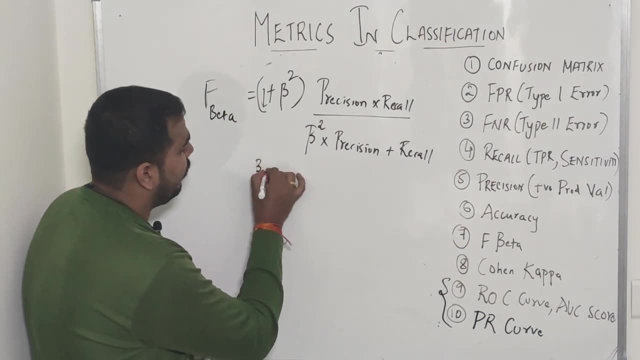 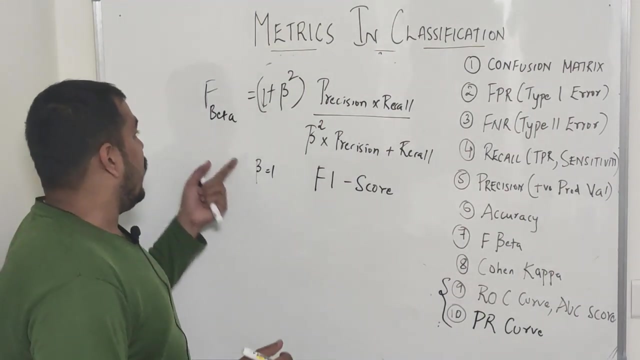 okay, Now how we should go ahead and select the beta value, I'll just tell you in a minute. but just understand one thing, guys: this exactly: if I just consider my beta value is 1- okay, This basically becomes an F1 score. okay, This basically becomes an F1 score. How to select: 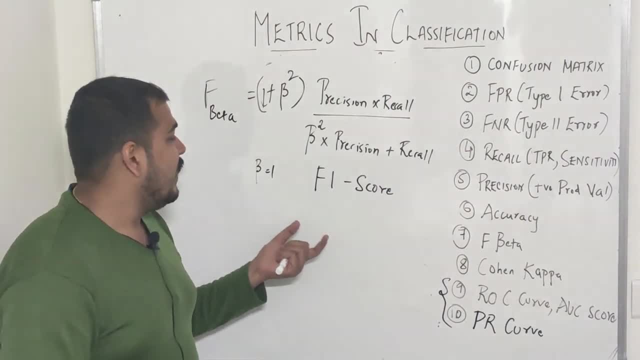 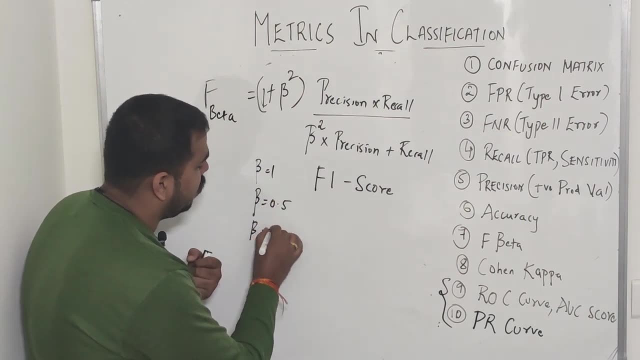 when to select. beta is equal to 1. I'm just going to tell you in a while. Similarly, beta values can vary. it can also be less than 0.1, it can be 0.5, it can be 2. you know, If it is 0.5, we basically. 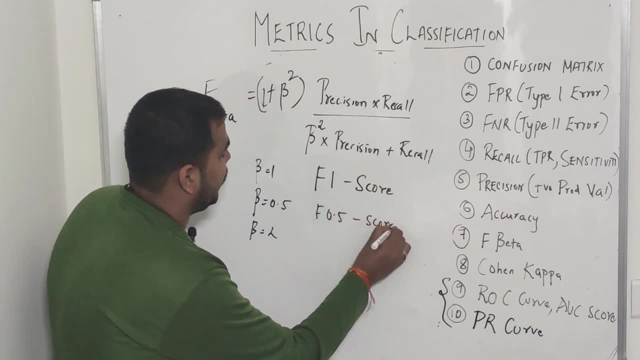 say this as F 0.5 score If it is 2, which basically say that F 2 score. okay, Now, if we say F 0.5 score, we basically say that F 0.5 score. If it is 2, we basically say that F. 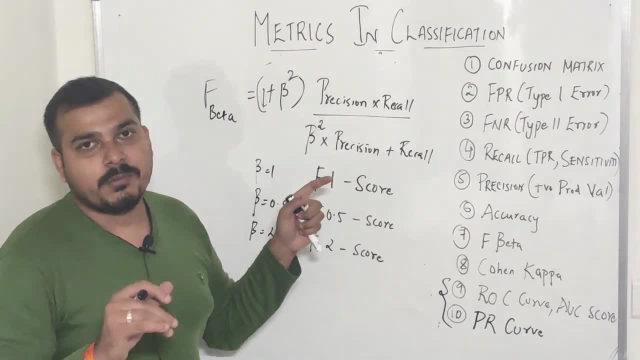 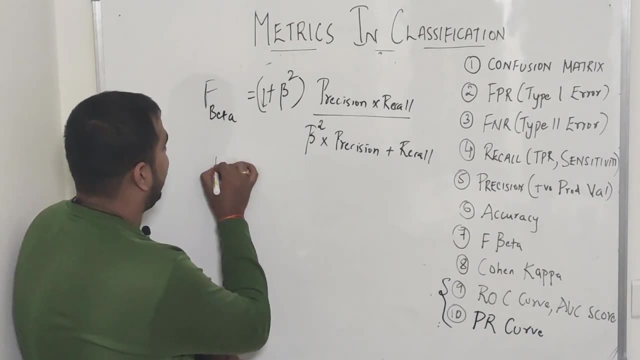 0.5 score. Now I hope you- I don't know whether you have seen this particular formula, guys, but just understand- this is my F beta and initially we need to select this particular beta value. Now consider that if my beta value is 1. Now this formula basically becomes 2 into precision. 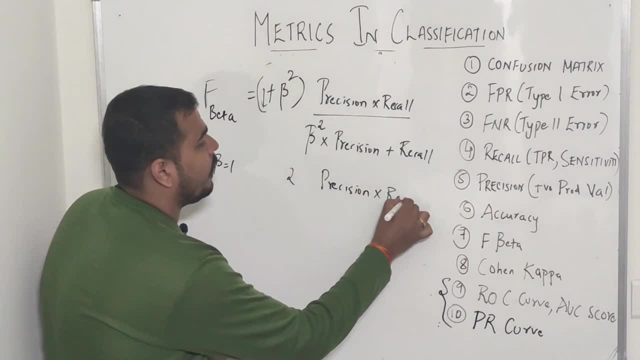 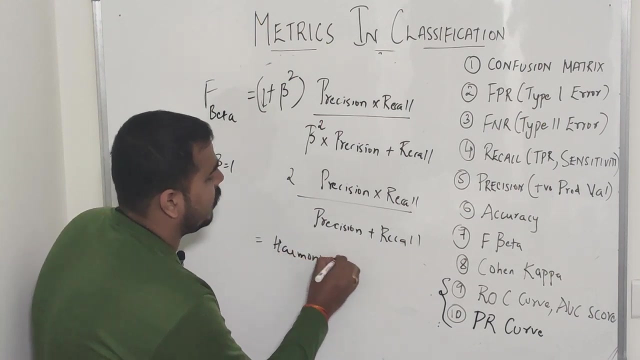 multiplied by recall, divided by precision plus recall. okay, and this is basically called as a. if you don't know about this guy, this is called as a harmonic mean. Harmonic mean: If I replace this precision recall by x and y, so this will become 2xy divided by x plus y. I hope you have been. 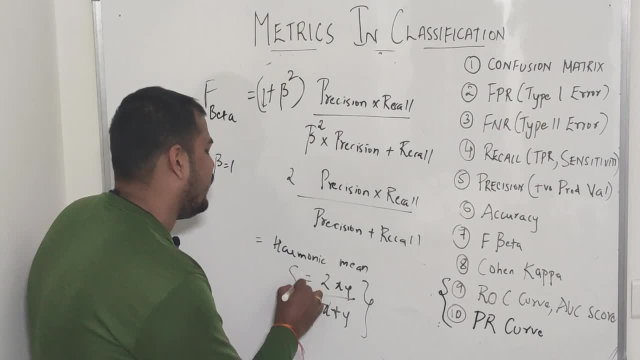 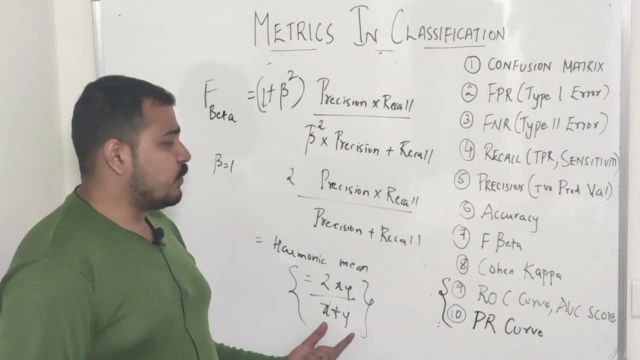 familiar with this particular formula itself. This was we used in some of the linear algebra in your school days and in your college days. if you remember, 2xy divided by x plus y- I'm considering precision- and x, recall as y precision. over here are x, x plus y. okay, 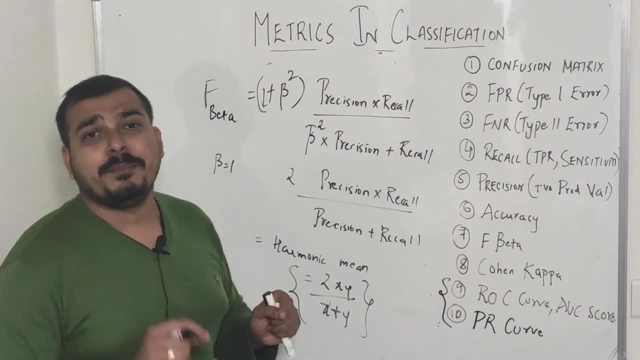 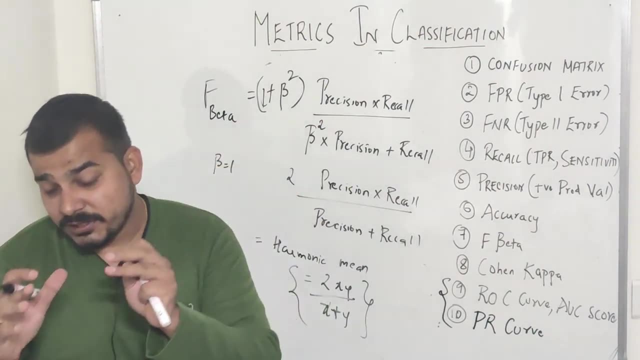 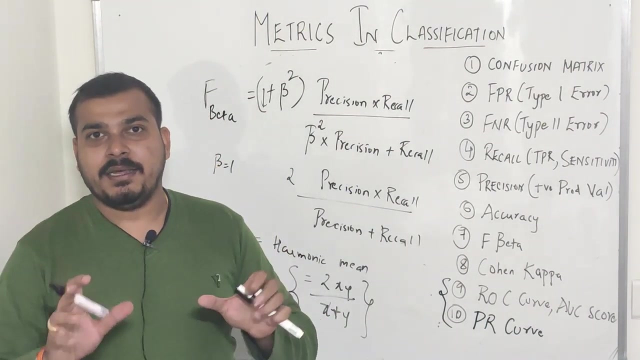 Now understand over here. when should we select? beta is equal to 1.. Now understand, guys, if you have a problem. statement where: wherever true positive- sorry, not true positive, false positive and false negative, both are equally important. Both are having a greater impact At that time. 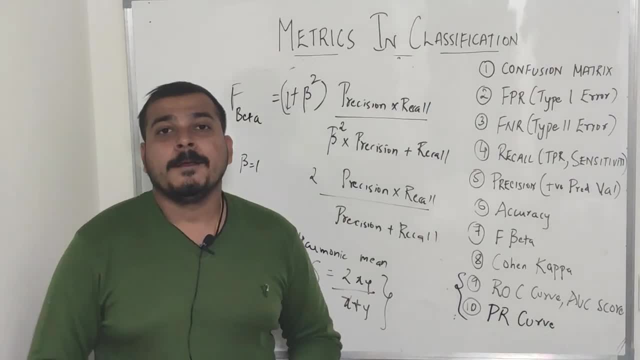 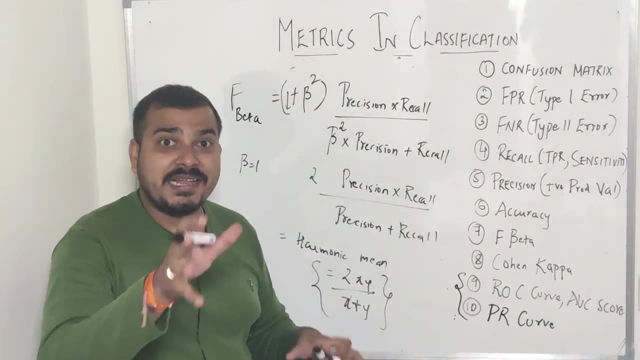 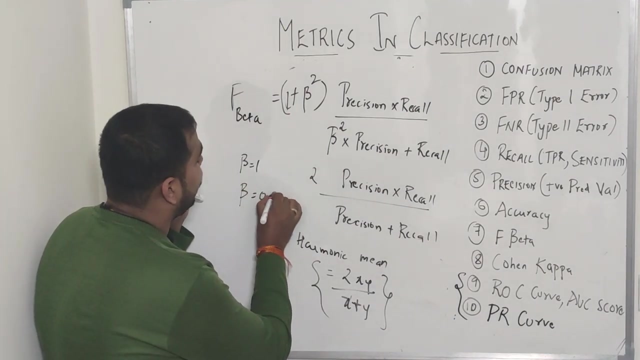 you go and select beta is equal to 1. okay. Now, in some of the scenarios, suppose your false positive is having more impact than the false negative. that is then the type 2 error. Okay, false positive is the type 1 error. At that time you reduce your beta value to 0.5 between 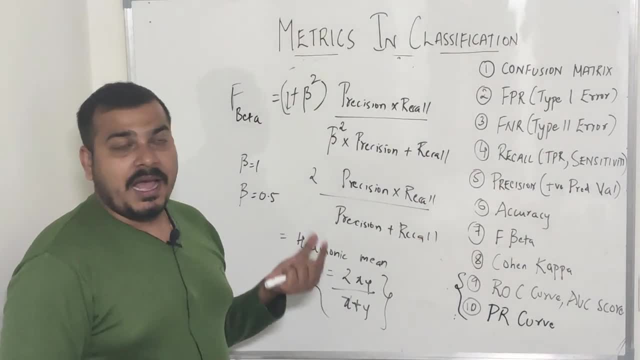 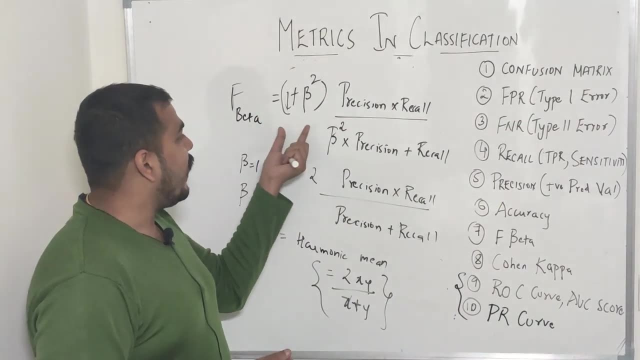 between 0 to 1.. Usually people select it as 0.5.. At that time this beta value will get converted to 0.5, so it will be 1 plus 0.25.. This is nothing but 1.25 multiplied by precision. into recall divided. 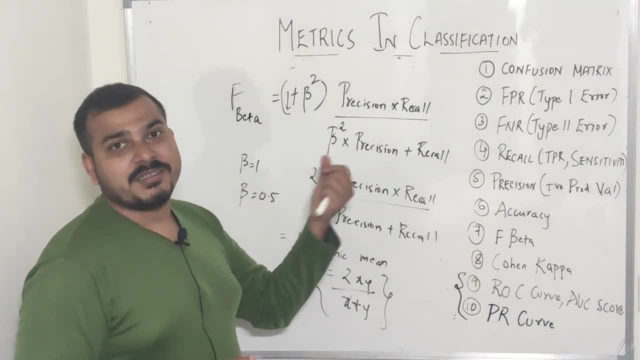 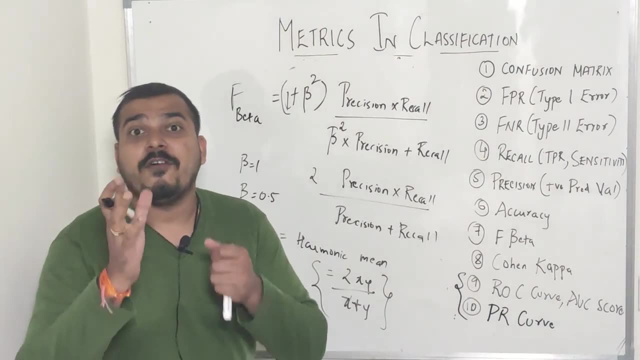 by this will basically become 0.25 into precision plus recall. So whenever your false positive is more important, we reduce this beta value. Now, if you have a problem, statement where false positive is higher than 0.25.. Now, similarly, if my false negative is high, false negative impact is high, right. 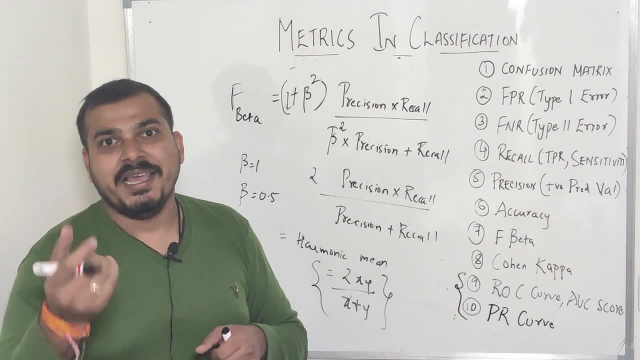 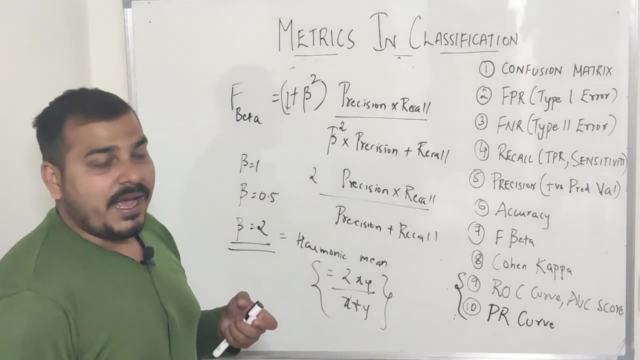 That is for recall, If you remember guys. okay, if that is high, at that time we specifically increase my beta value greater than 1.. Suppose I consider it as 2, right, At that time, what will happen again? I will try to apply in this beta value this particular 2 value. this will nothing be, but.